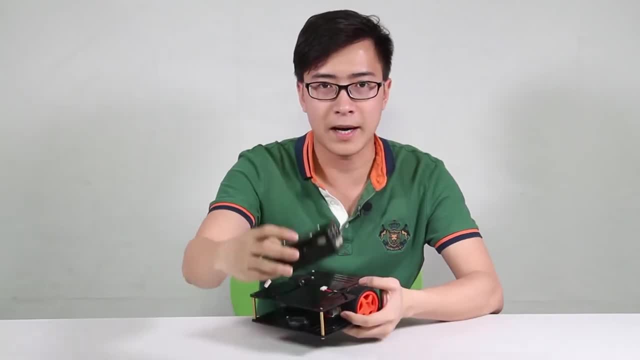 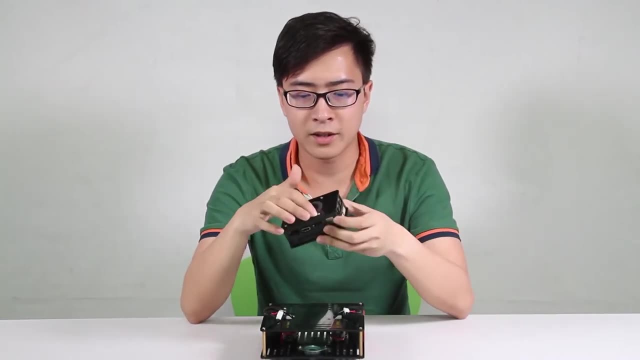 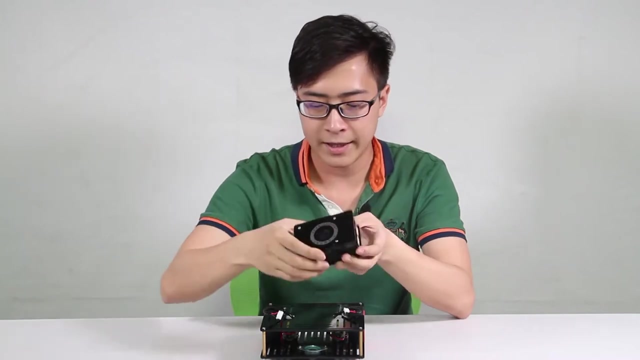 the Pi smart car is combined of two things: the Pi smart and the car. The Pi smart is a smart robot platform we build with speech interface based on Raspberry Pi, so that's why we need a Raspberry Pi 3 and the car is just a simple. 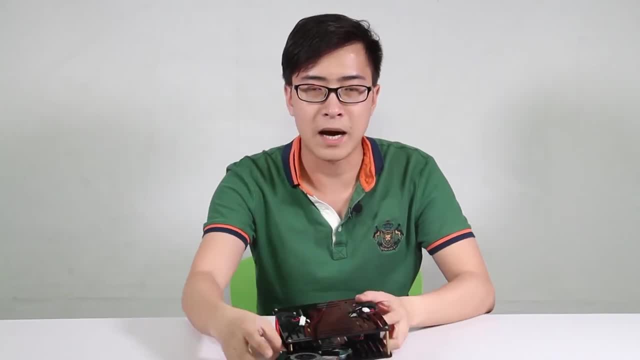 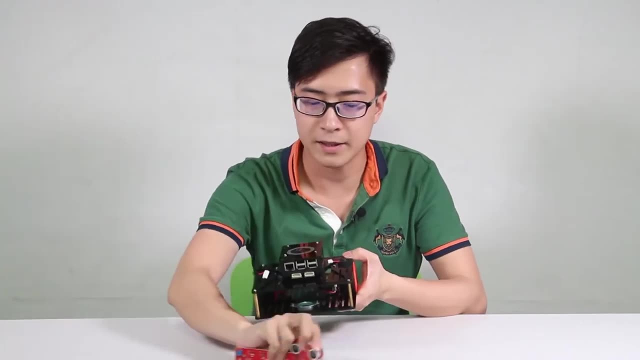 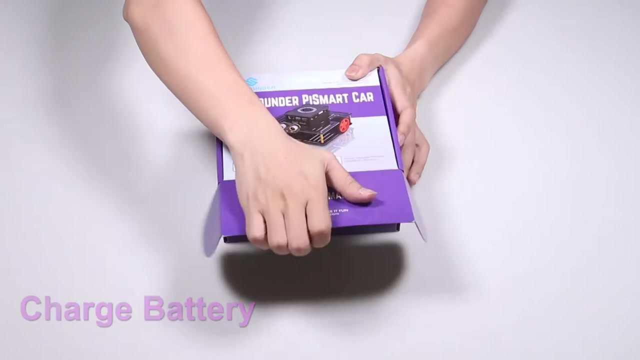 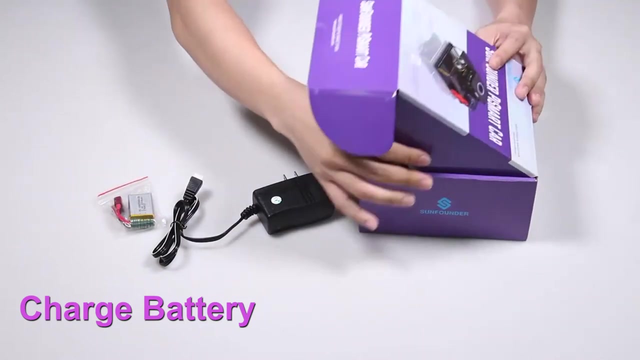 three-wheel car with two motors, so the Pi smart car is combining two things together and has some more sensors. As soon as you get that clear, we can now begin. Let's open the box and here's the battery charger and the battery. The battery charger looks. 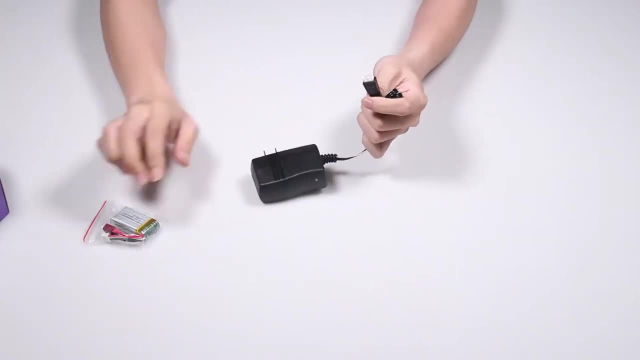 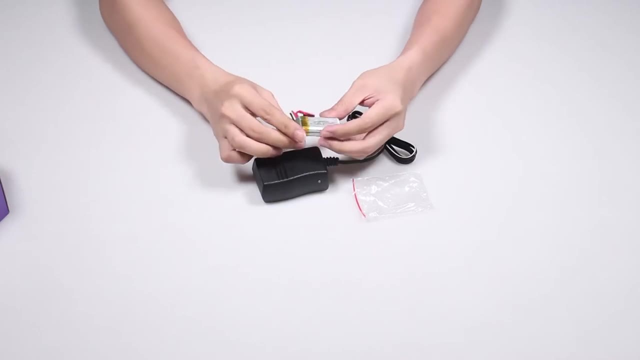 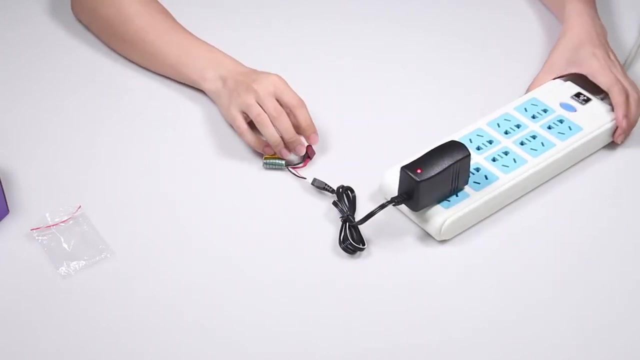 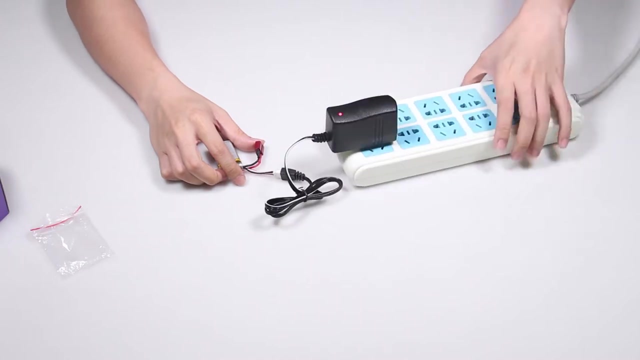 like a power adapter with such head and the battery is a 7.4 volt 650 mAh battery. Connect this while it jacks and plug onto the wall. You can see the LED light is red here and it would turn green. after it's done charging, Let's put. 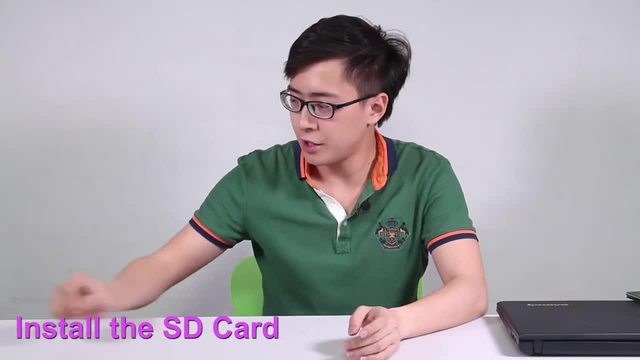 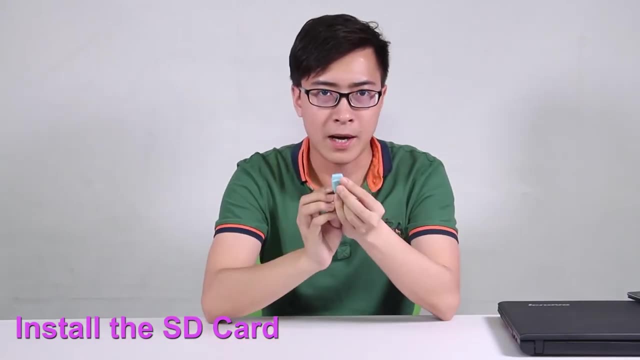 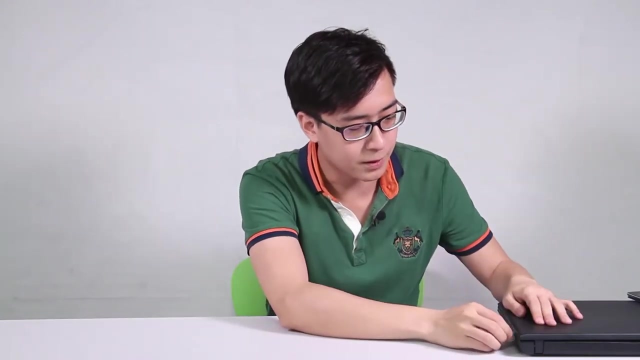 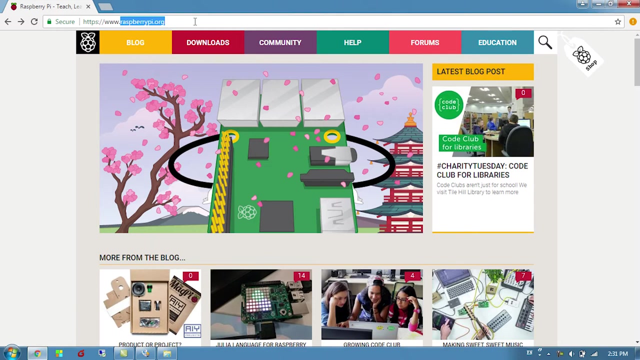 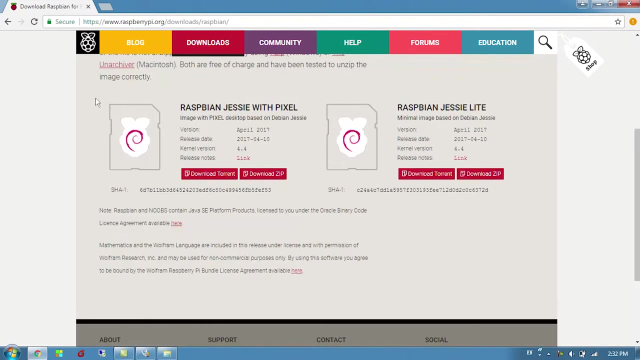 it aside While the battery is charging. you can now set up the micro SD card. Plug the micro SD card into a USB micro SD adapter. Then plug the adapter into your computer. Download the latest Raspbian from raspberrypiorg: Go to download Raspbian and here download. 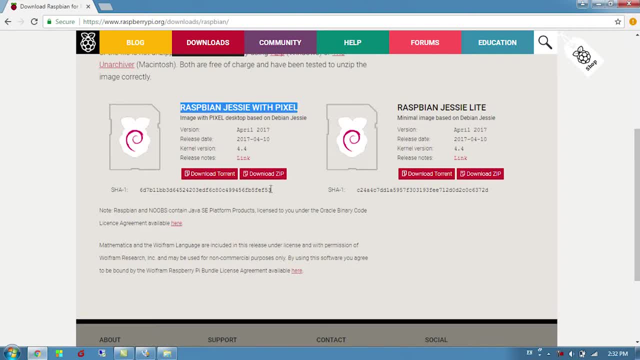 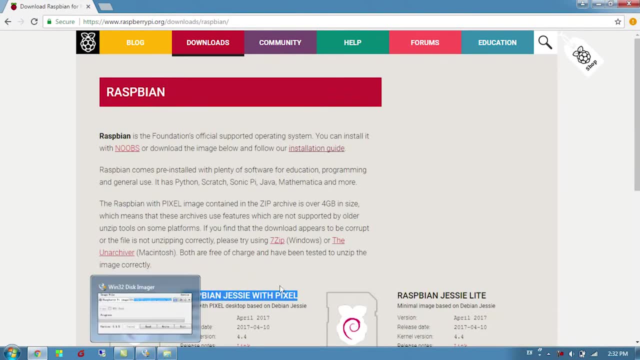 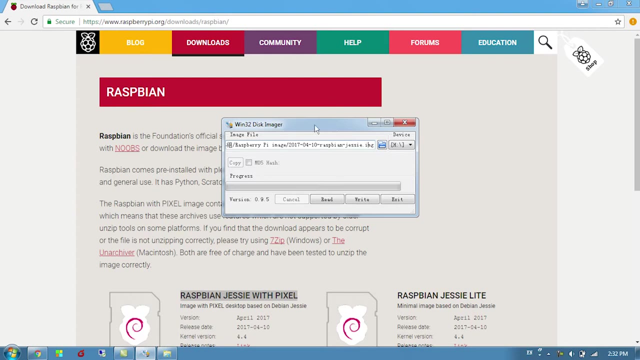 this Raspbian Jessie with Pixel and download this IP and, after downloading, unzip the zip file and got an image file and use this win32 disk Imager, Choose your SD card and hit write and then, yes, I have already burned the image, so I'm gonna skip this, If you. 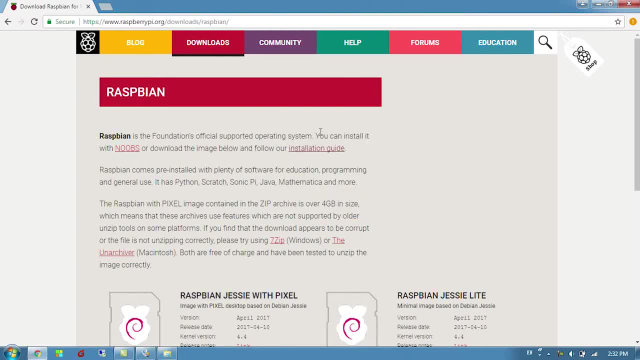 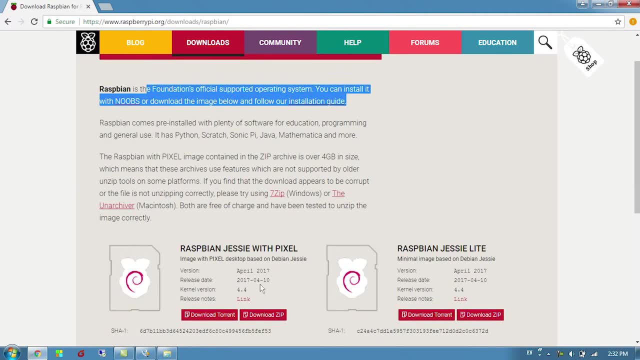 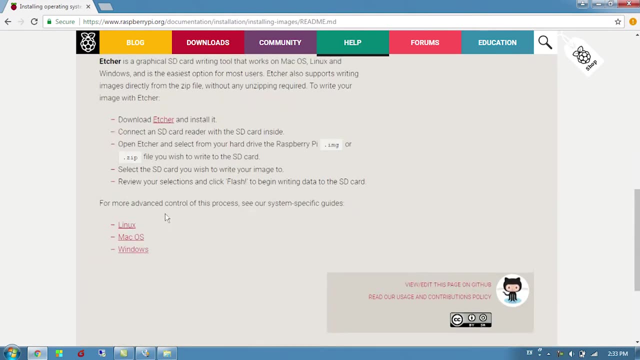 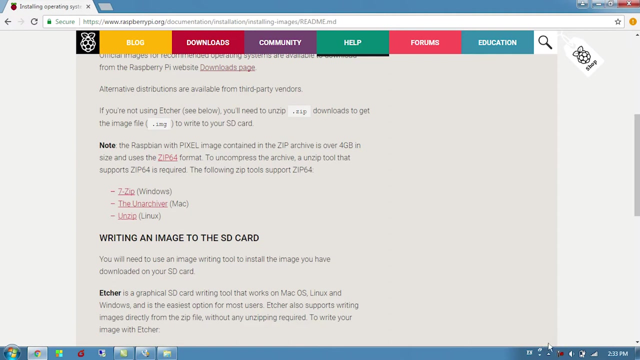 are using the other platform or anything, or you need a detailed installation guide. you can check this. It's just above this download page here installation guide. You can get all the platform and every details. So after you have done burning the image, you can unmount the SD card. 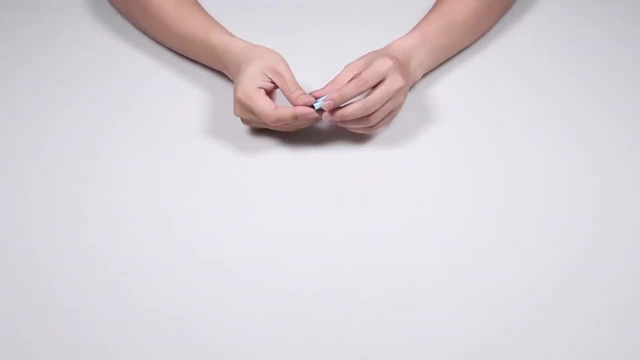 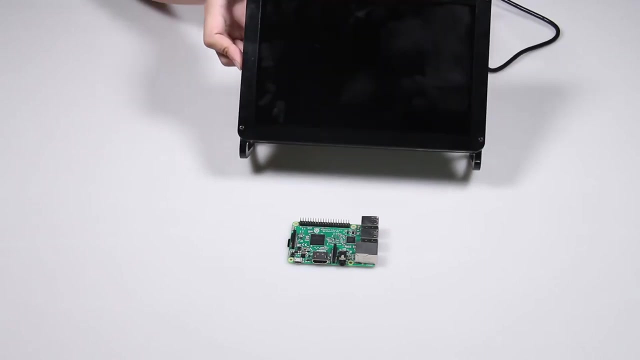 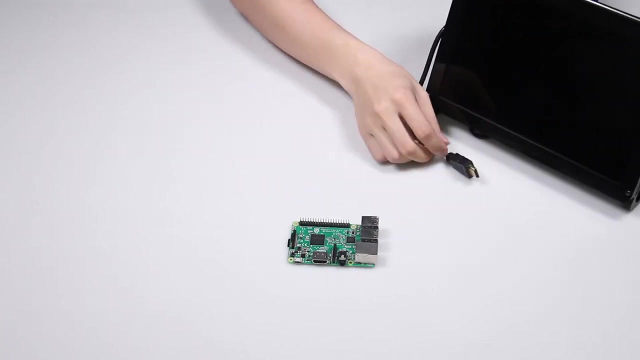 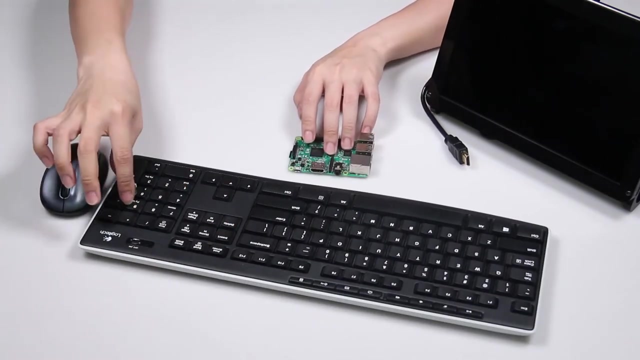 eject. Now take the SD card from the card reader and plug the SD card into the Raspberry Pi 3.. Then you also need a HDMI port monitor with the HDMI cable, and you also need USB keyboard and mouse. I got here a wireless one. Plug the USB. 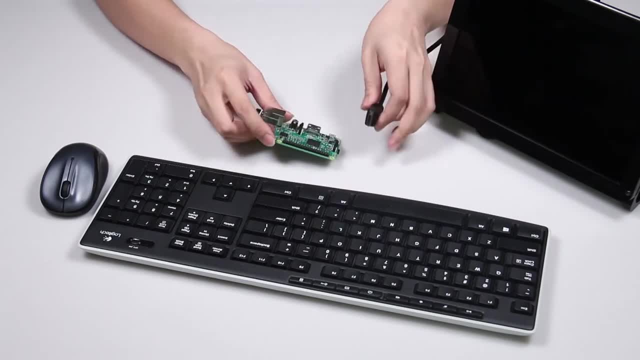 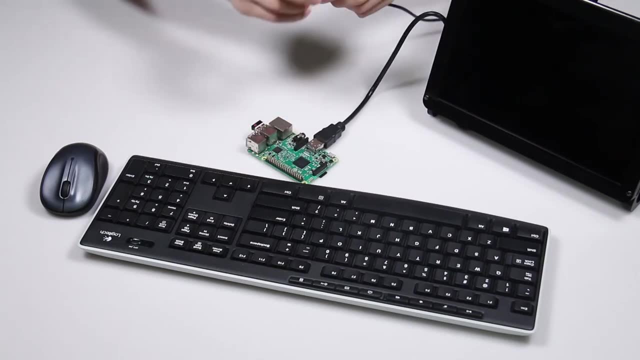 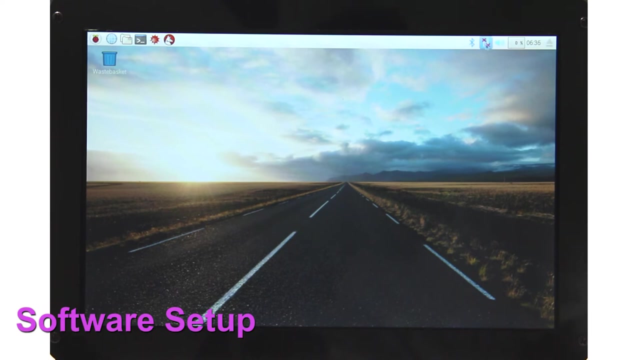 keyboard and mouse into the Raspberry Pi and also HDMI cable, Then power the Raspberry Pi. We are going to set up software first. After the Pi is booted up, choose the top right corner of this red cross on it and find your Wi-Fi SSID Type in the password. Then it's linking here After. 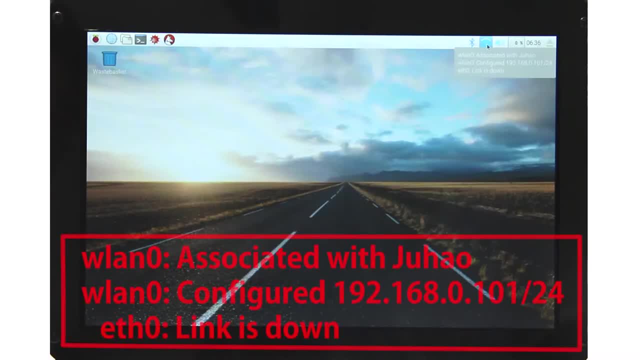 it's connected. you can point to this icon and see the IP address of your Raspberry Pi. Here you should see the IP address of your Raspberry Pi. Here you should see the IP address of your Raspberry Pi. Here you should see the IP address of your Raspberry Pi. 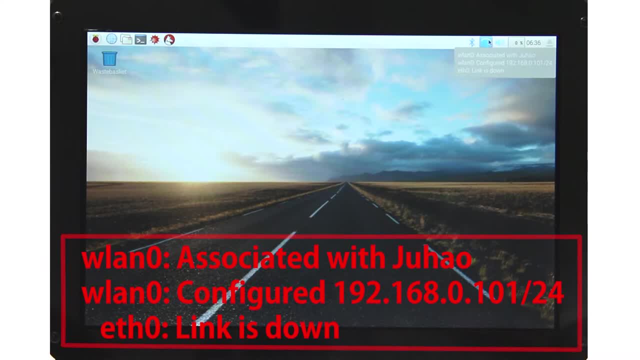 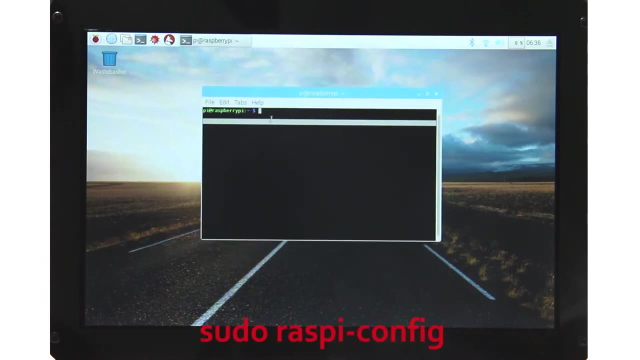 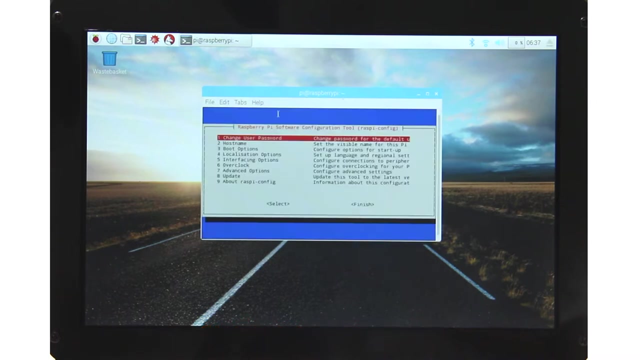 Note it down: My IP address is 192.168.0.1.101.. Okay, then open this terminal icon. Open terminal and type in sudo raspi-config In this raspi-config interface. go to interfacing option and SSH. Would you like to enable? Choose yes and it will. 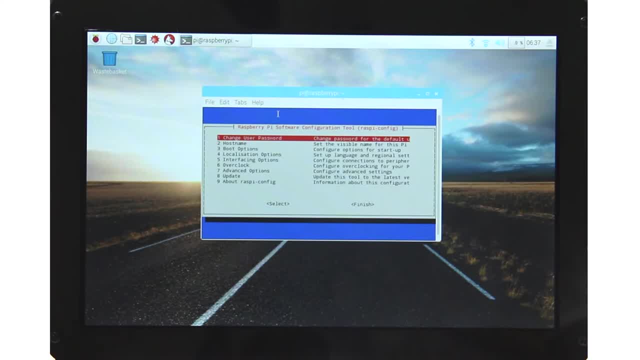 enable the SSH so that we could remote connect to the Raspberry Pi. Then you can also do the other changes, like change your user password and change the host name or the. in localization options: Here you can change your keyboard layout. In localization options: here you can change your keyboard layout. 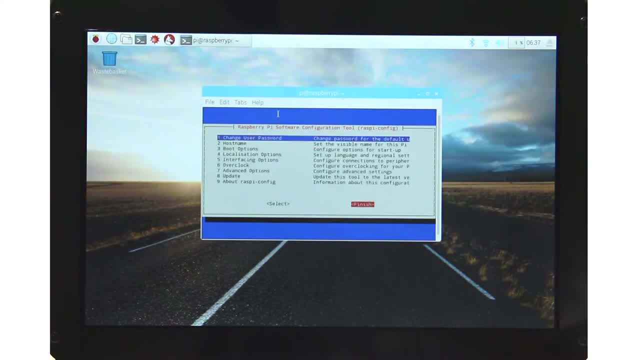 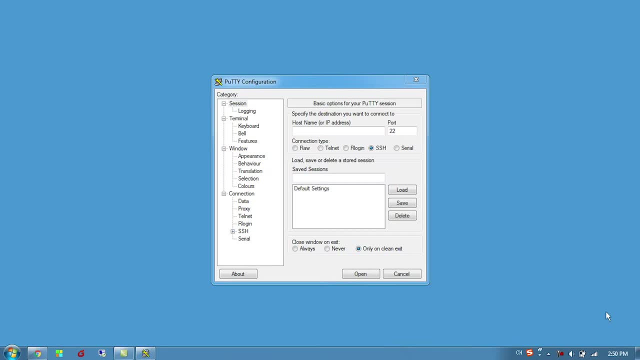 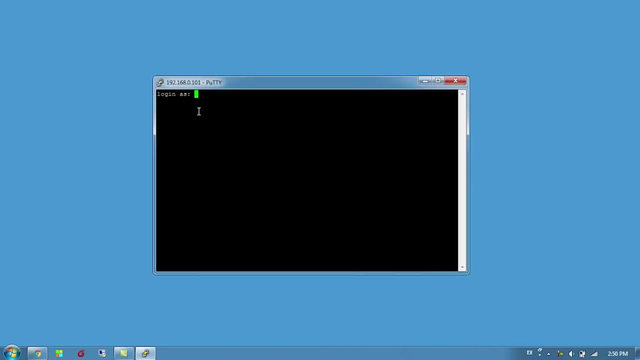 In localization options. here you can change your keyboard layout. Then hit back and finish. Then on your PC open PuTTY. Try to remote access to the Raspberry Pi In section type in the IP address you just noted down and click open. It worked. It prompt login as type in Pi. 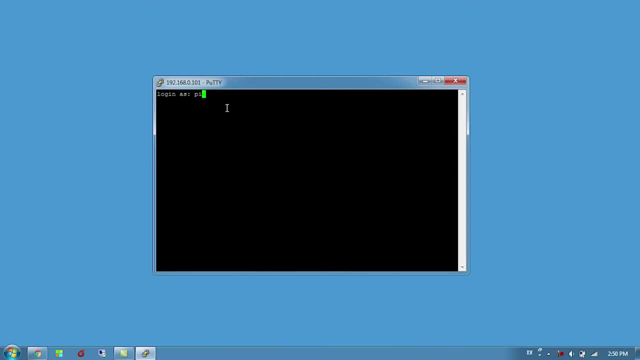 It worked. It prompt login as type in Pi As the Raspberry Pi's username and default password, if you didn't change it Raspberry. Okay, now we need to install the software. Download the Pi smart repo from GitHub with git clone https Sorry. 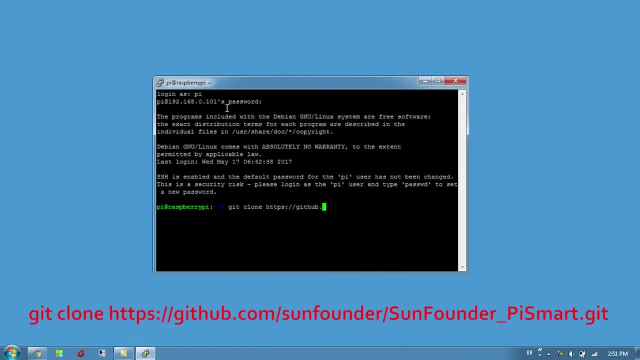 https. githubcom. slash some founder slash some founder pi smart dot git. The command will be in the description under the video, Then hit enter. I've already. The command will be in the description under the video, Then hit enter. I've already. 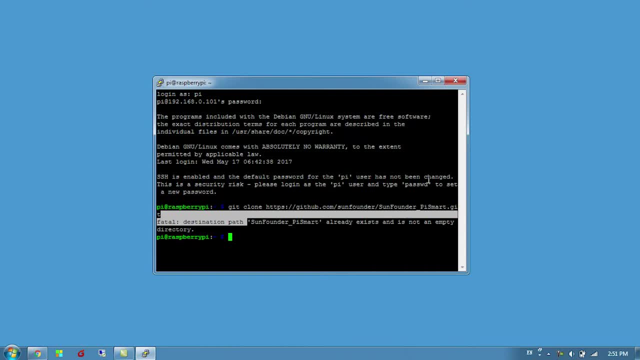 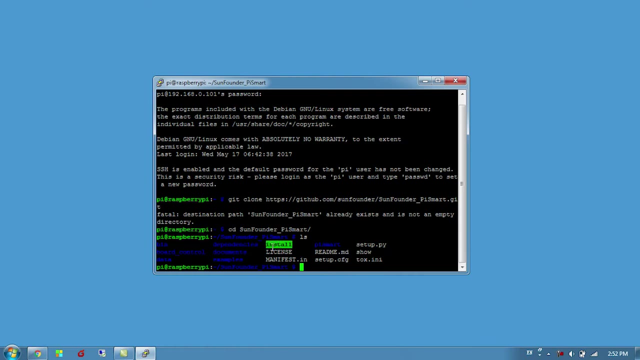 downloaded this because this might take some time. So let's move on to install Change directory. to some founder pi smart And we provide a super easy install script here. And so type in sudo dot slash install. And so type in sudo dot slash install. 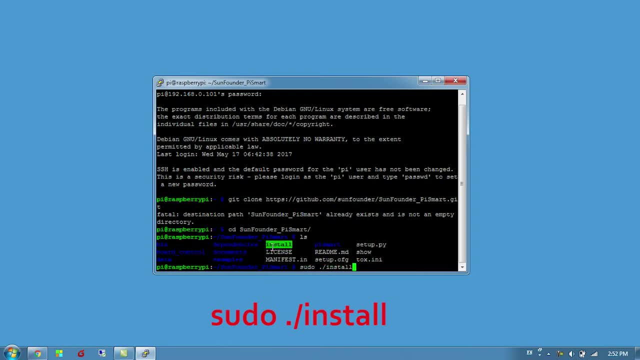 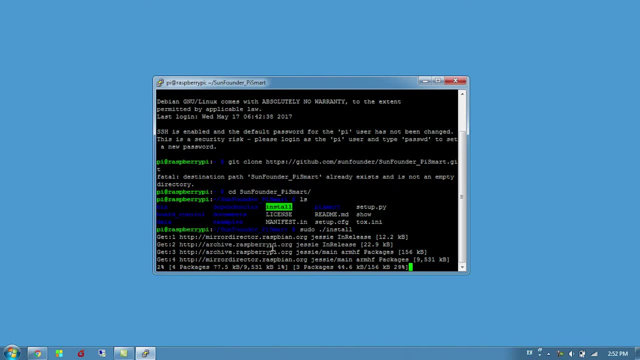 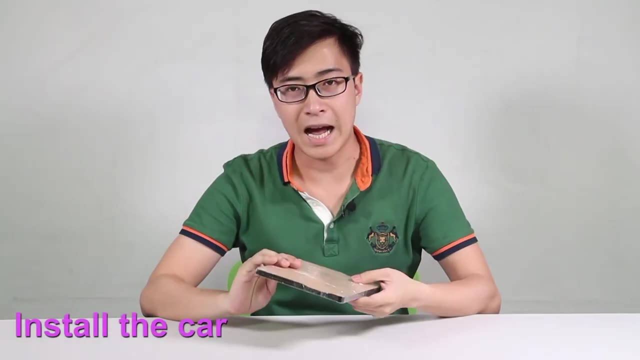 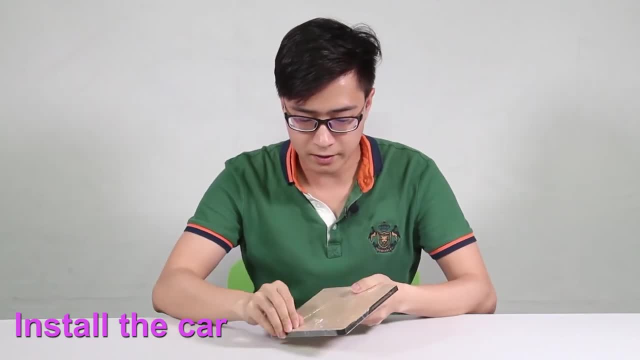 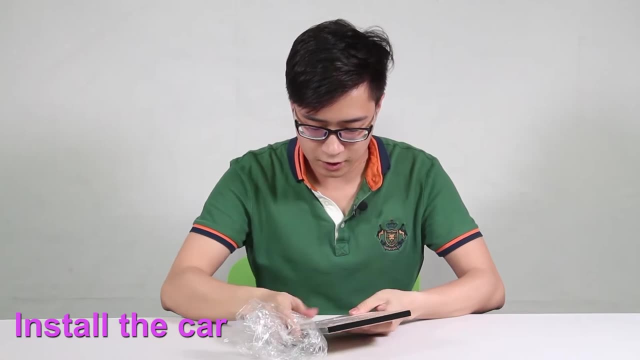 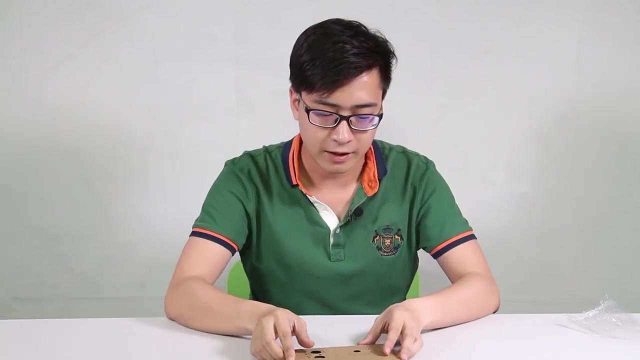 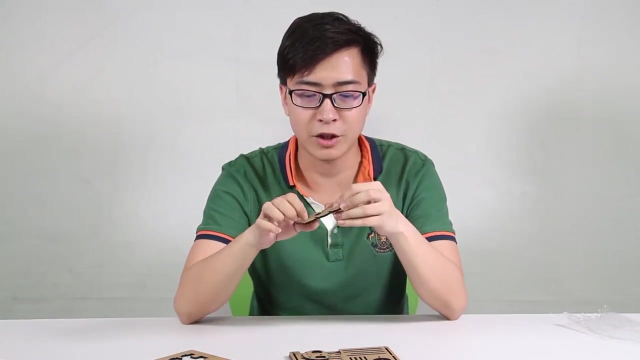 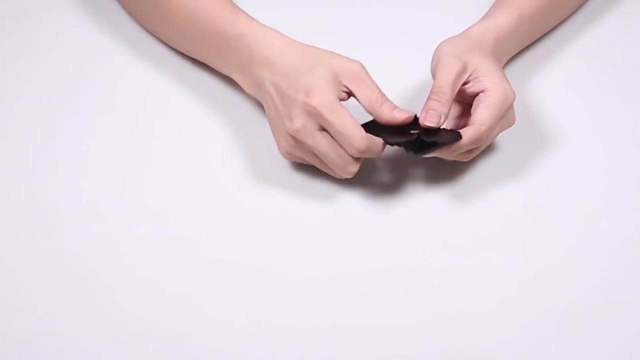 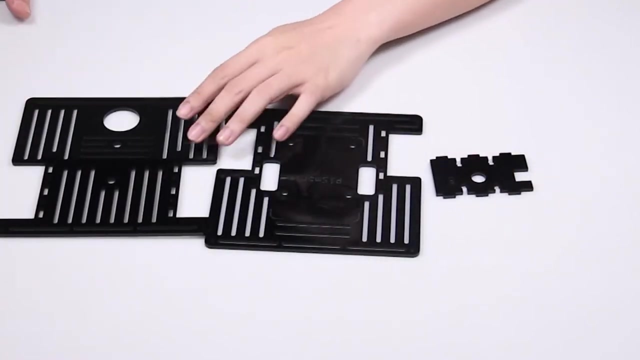 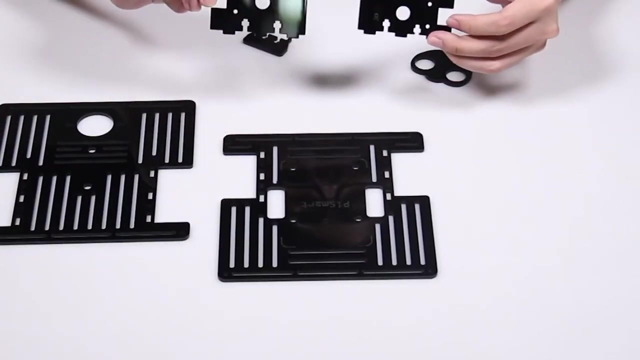 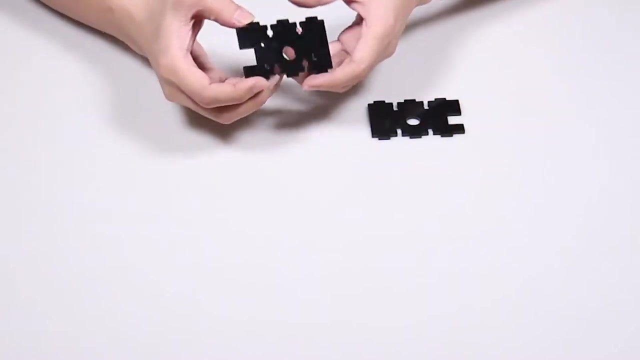 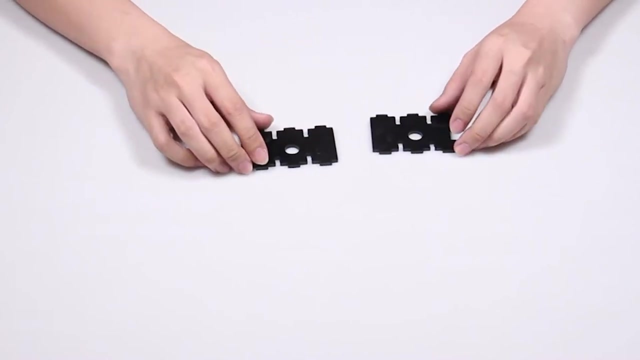 with PI smart car, unwrap it. the acrylic plate are always covered with papers or plastic to avoid the scratches, so you need to peel this off to give a nice look here. I have already done them both side. okay, now let's take these two pieces- the one mark with L and one mark with R- and take 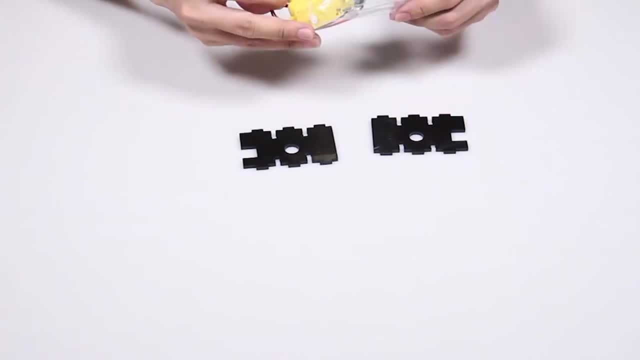 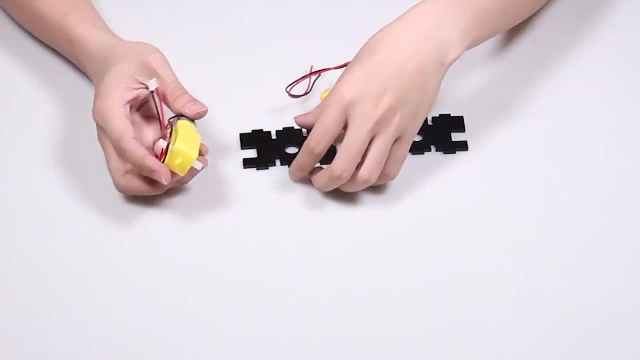 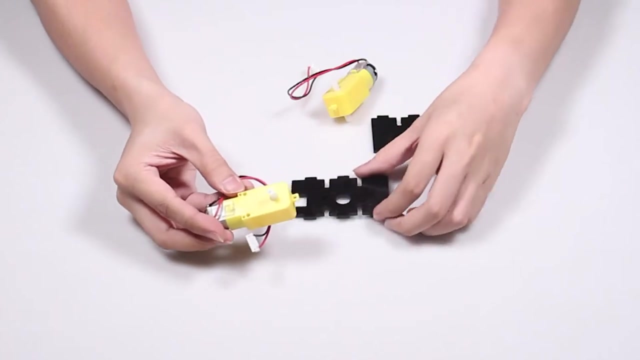 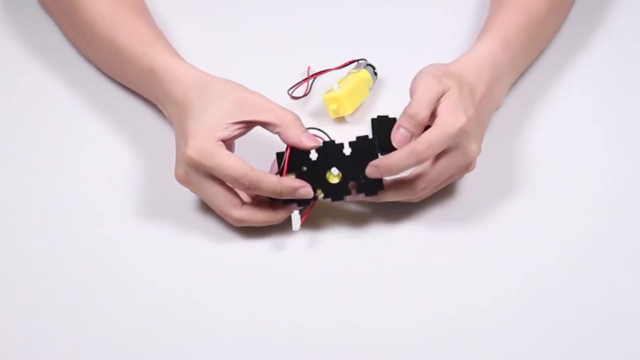 them both sides. okay, now let's take these two pieces- the one mark with L and one mark with R- and take. Take the motors here. we should mount them like this- you can see a knob here, this face is flat- and mount them like this. the label should face out and the wire goes to the board. 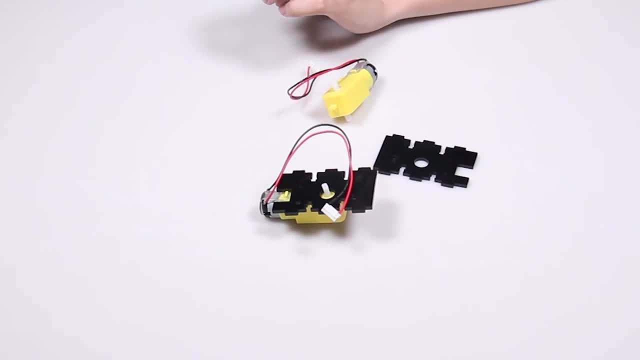 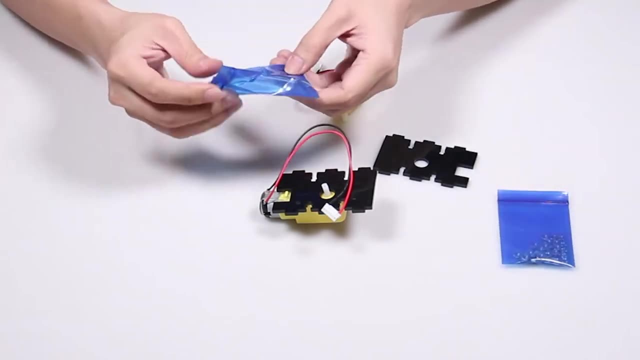 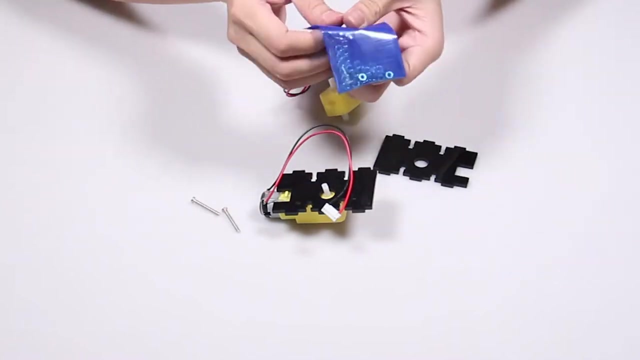 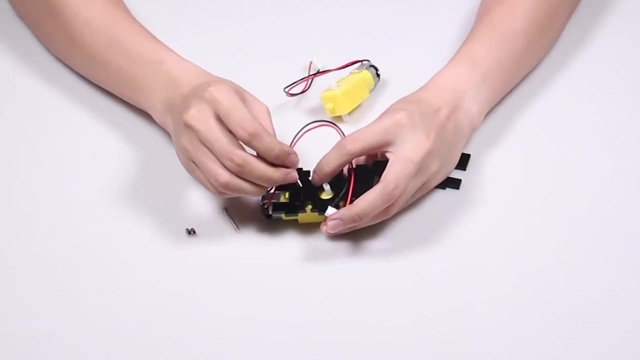 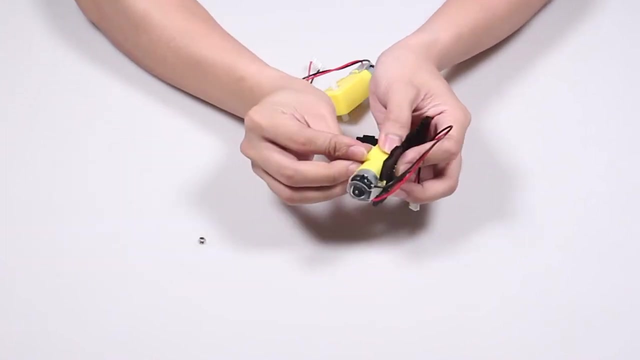 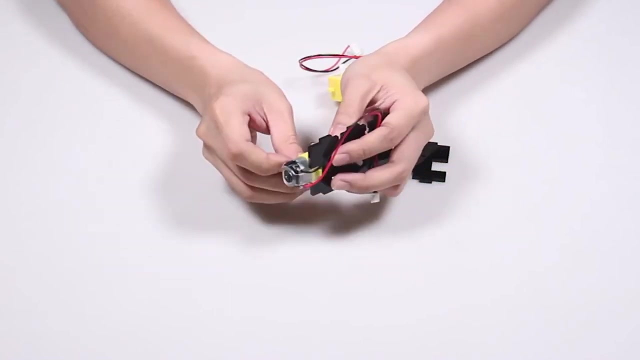 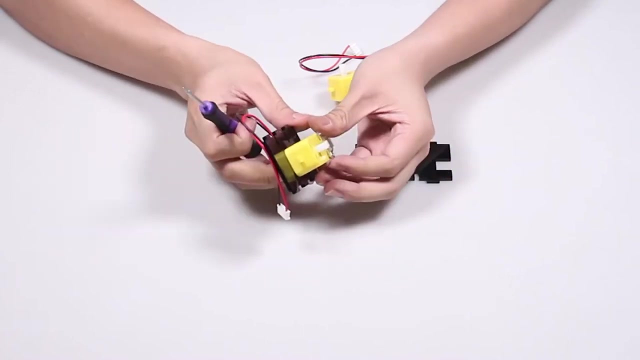 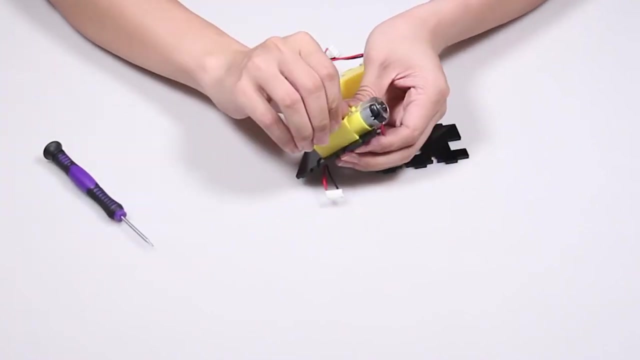 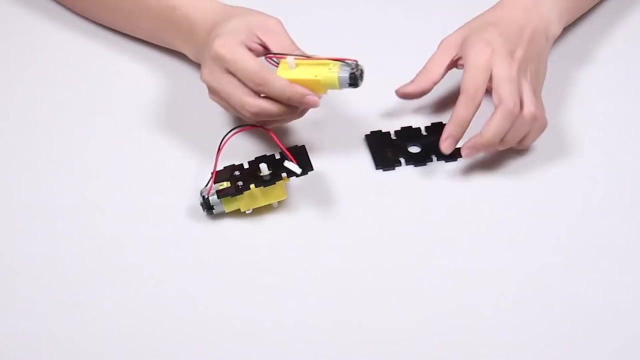 here and take out M325, the long screws and some M3 nuts. take two of the screws and two of the nuts Through the screws, like this, Like this, Like this, and tighten them when you finish. it should look like this and do the same. 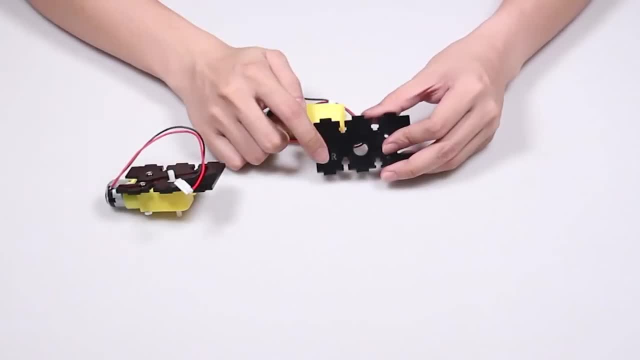 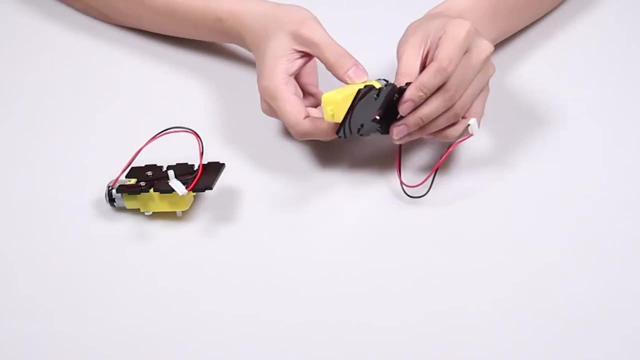 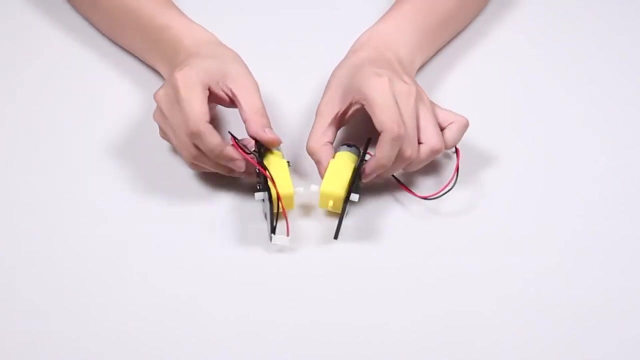 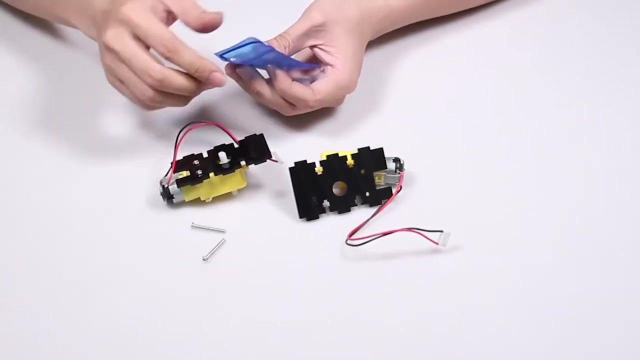 with the other motors the same: the label face out and then face with flat. connect it like this. it should be mirrored. like this: it should be mirrored. also, take two long screws and two nuts Like this, Like this: 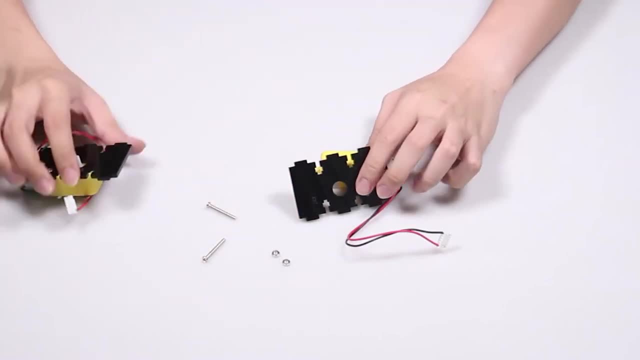 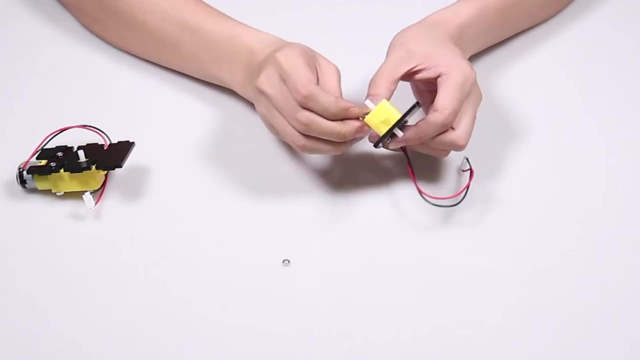 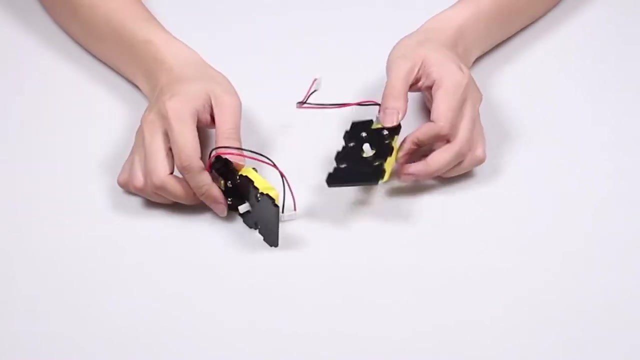 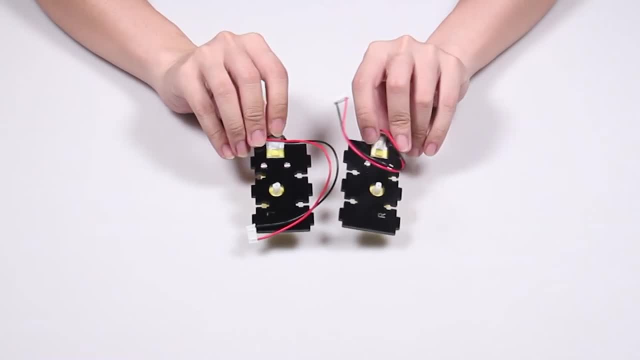 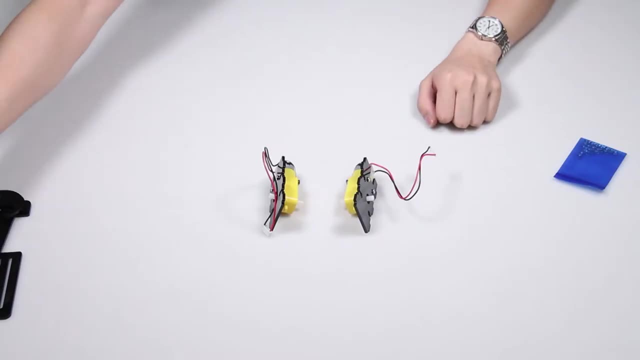 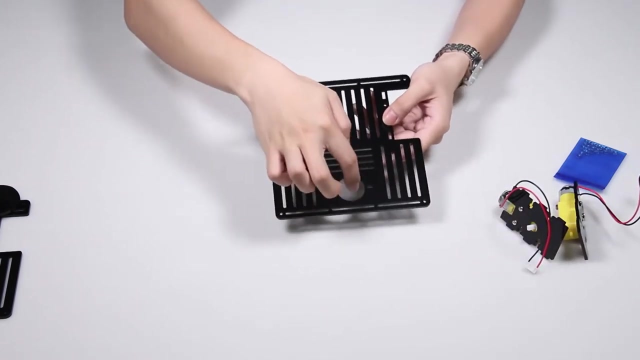 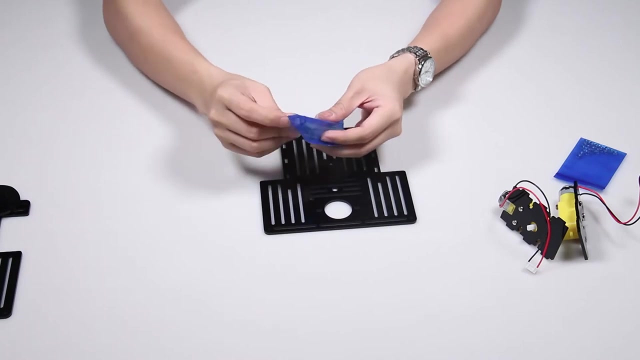 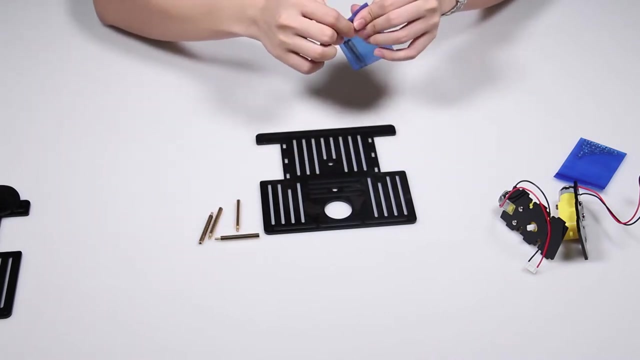 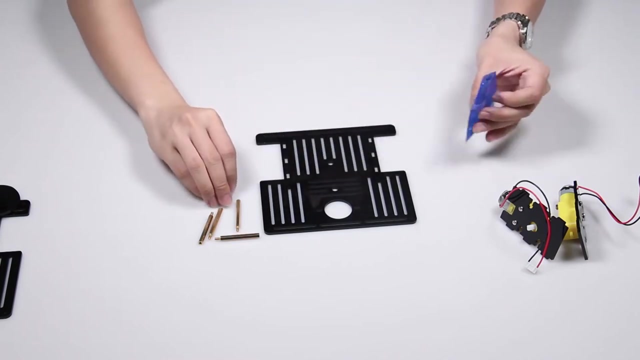 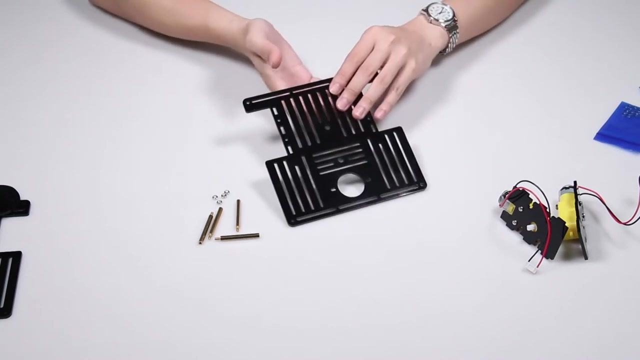 That's it. They are mirrored. Now take the bottom board. it should look like this: put it aside with a round hole here and mount the M340 copper standoffs, Long one with M3 nuts. you can see a logo here. it should be on the bottom. 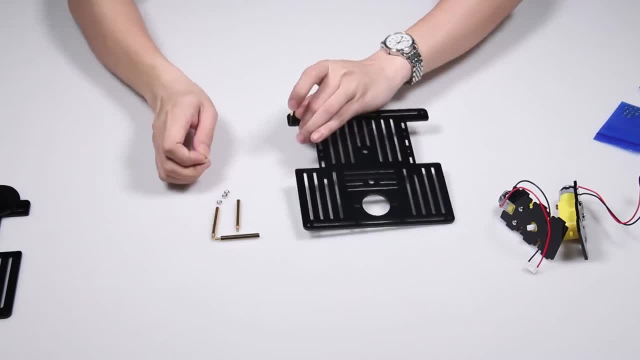 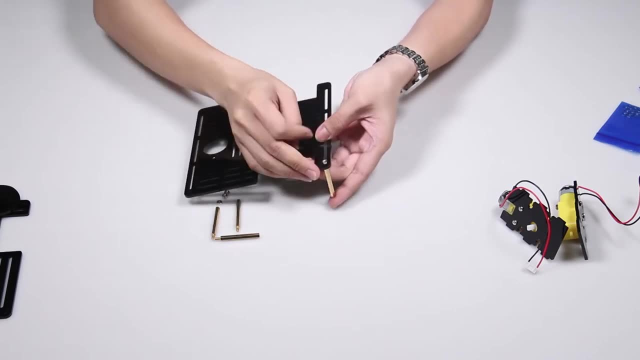 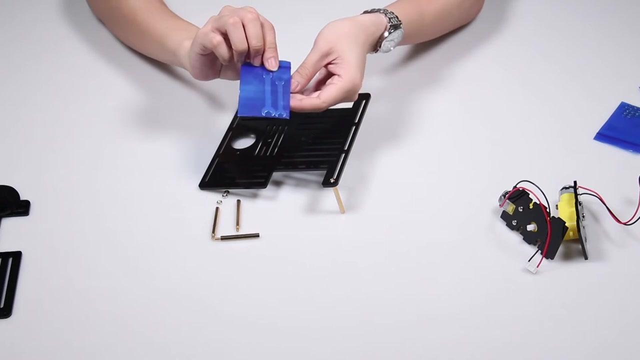 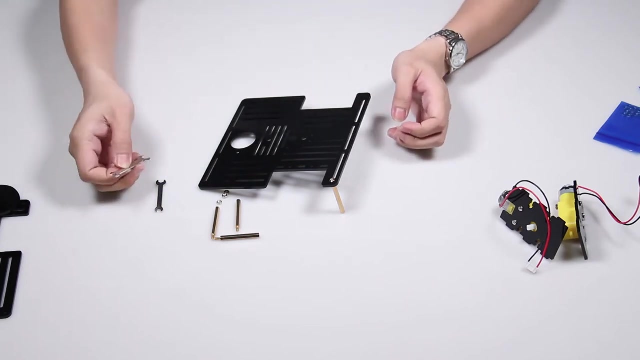 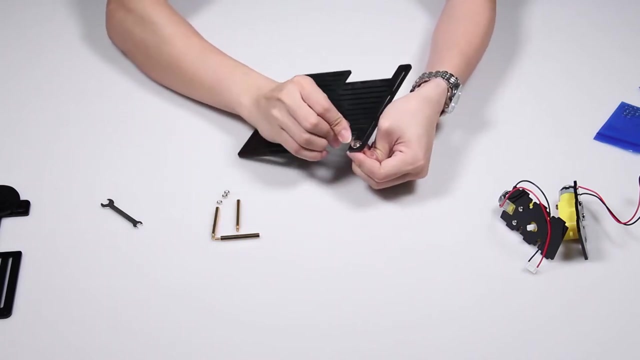 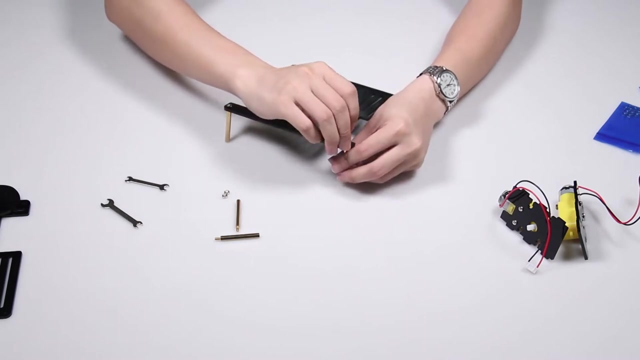 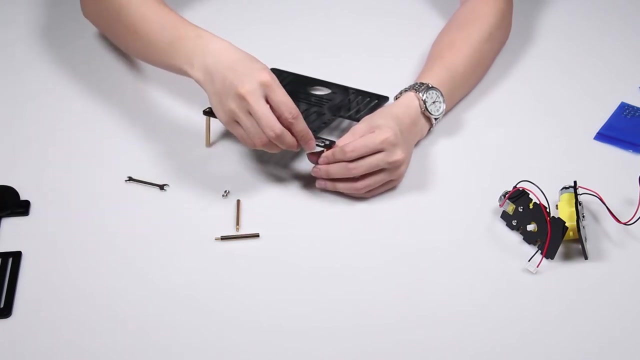 So the standoffs goes here. Tight it with the nuts. You can also use a wrench here. these are 4 sizes. this is a M3, this one. Tight it with a wrench here. these are 4 sizes. this is a M3, this one. 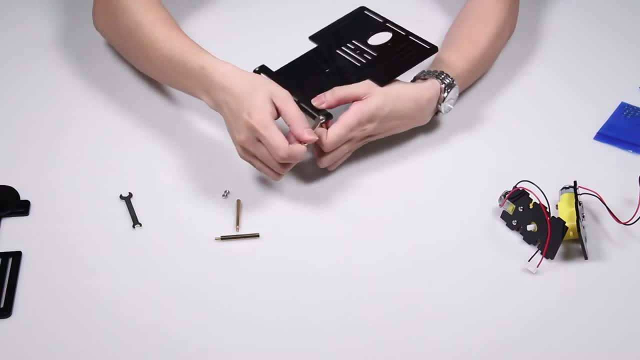 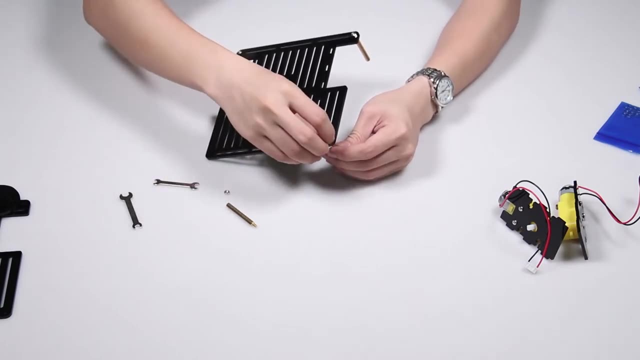 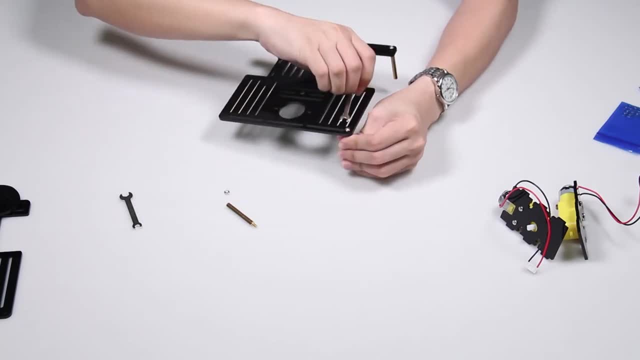 Tight it with a wrench here. these are 4 sizes. this is a M3, this one. Tight it with a wrench. here. these are 4 sizes. this one. Tight it with a wrench here. these are 4 sizes. this one. 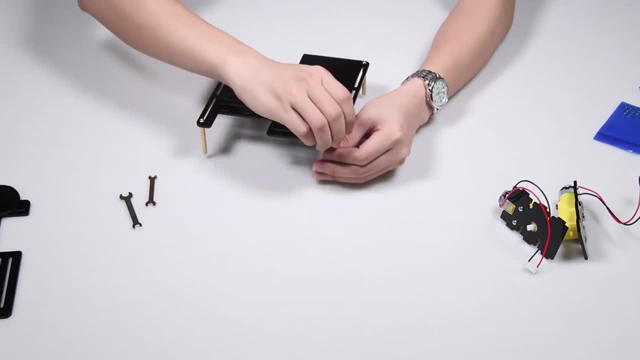 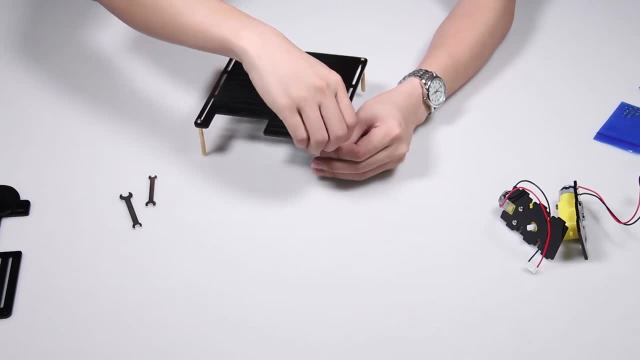 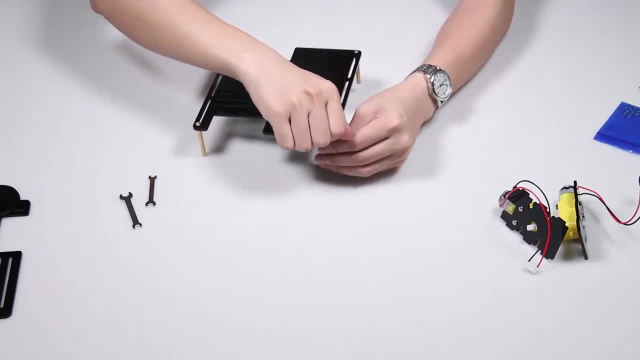 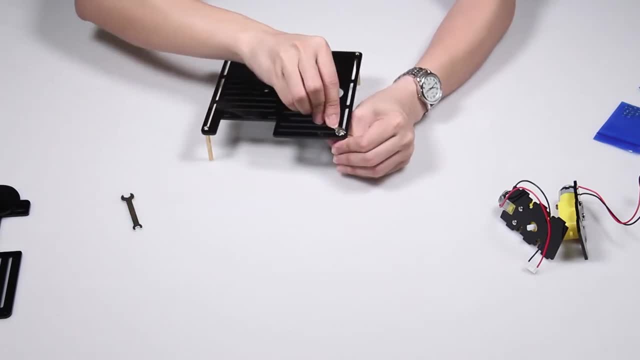 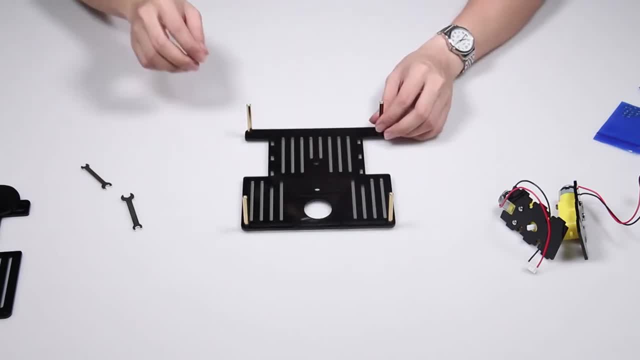 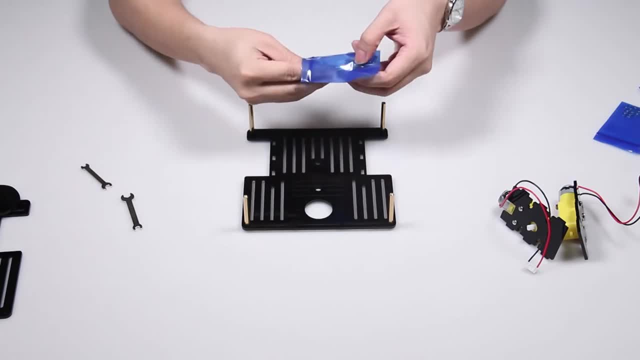 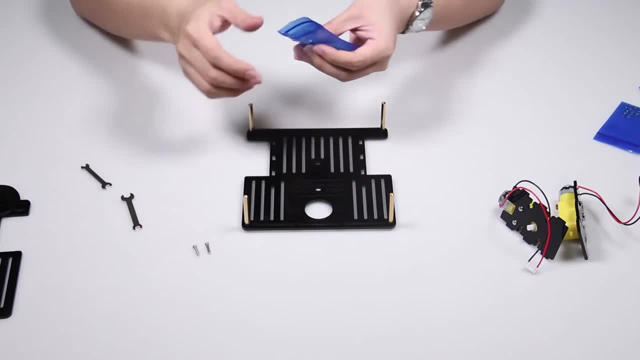 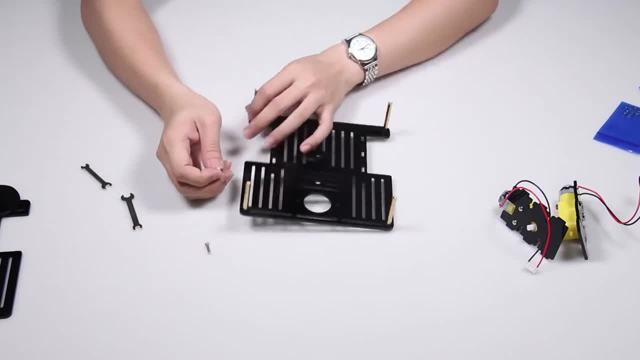 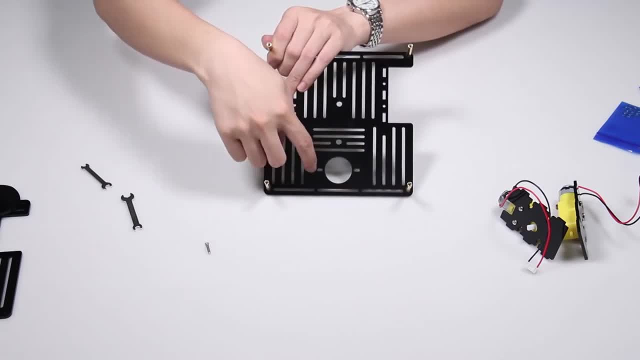 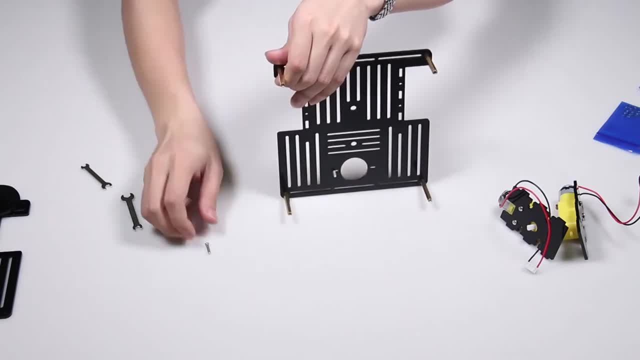 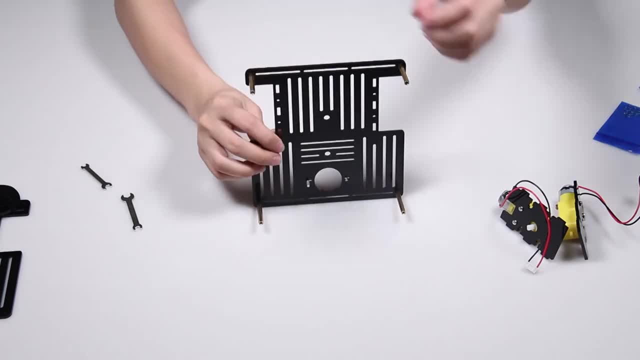 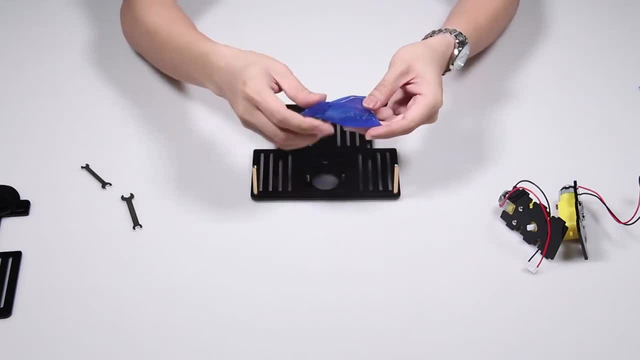 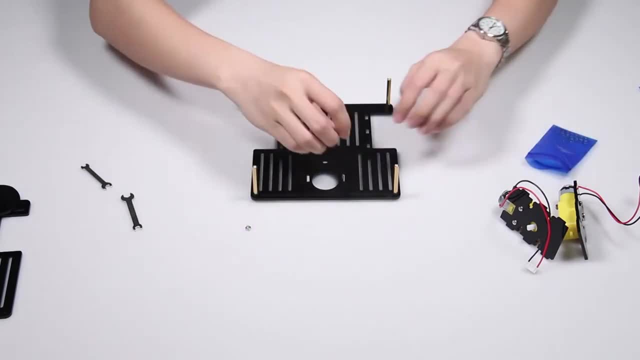 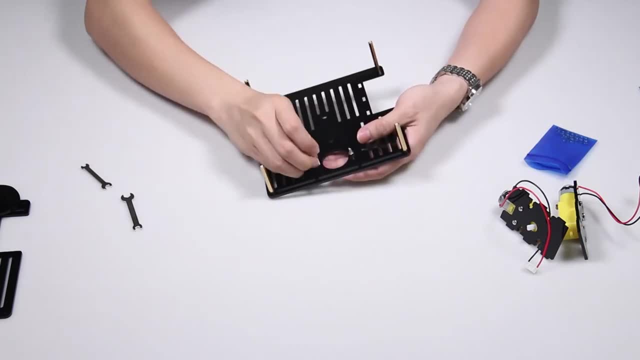 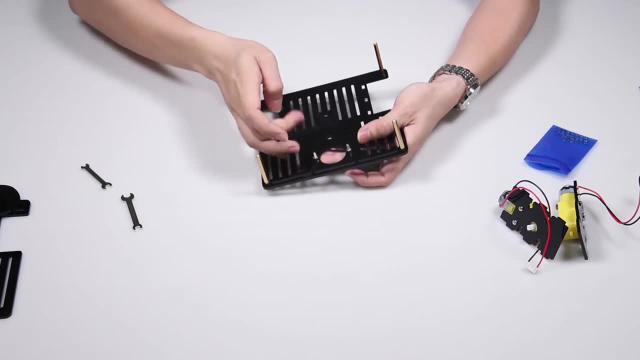 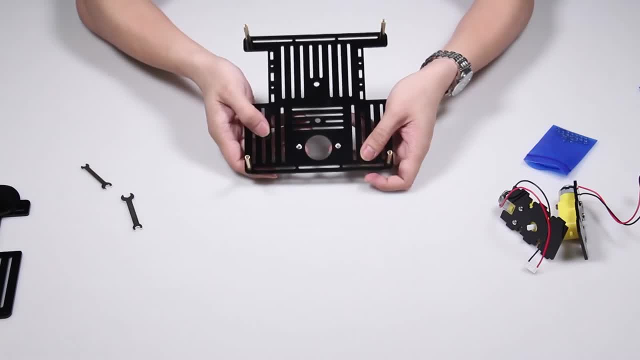 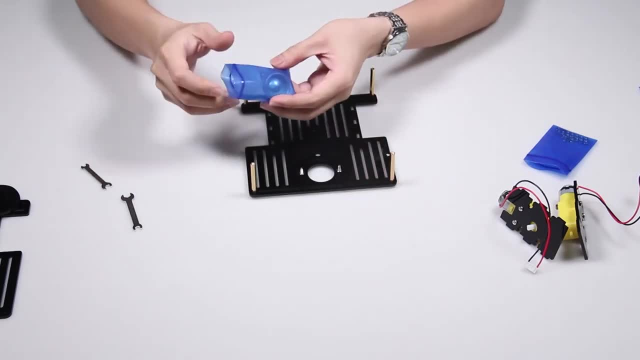 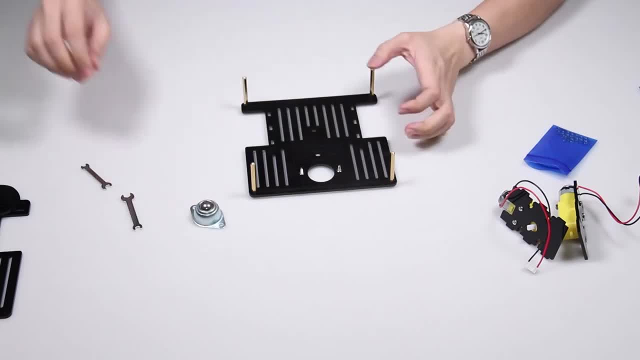 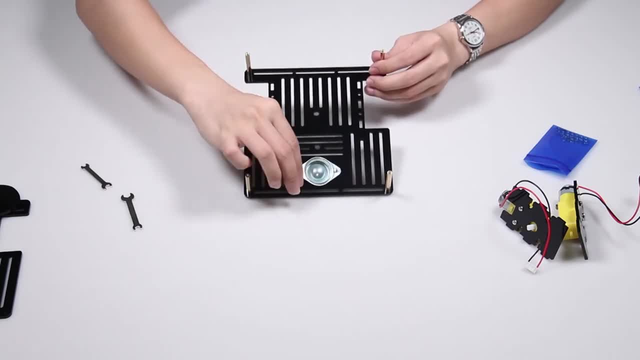 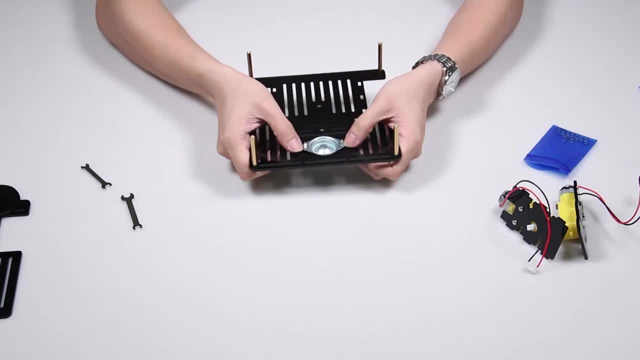 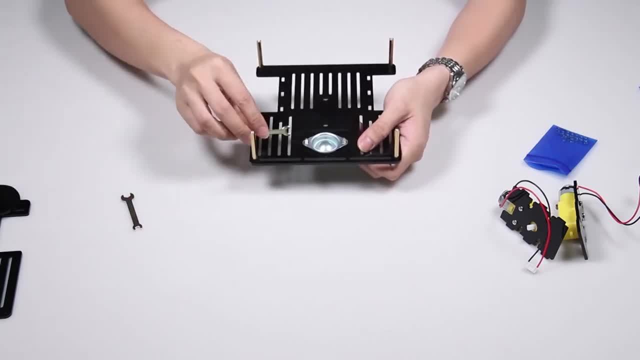 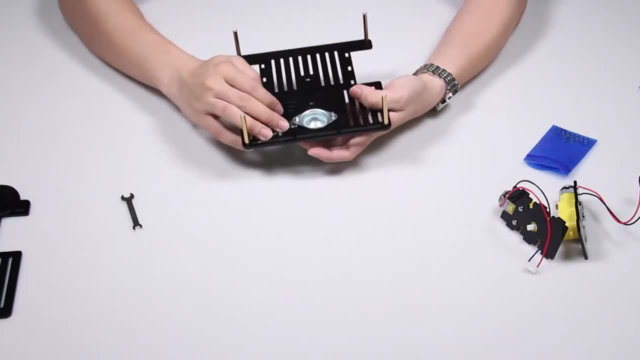 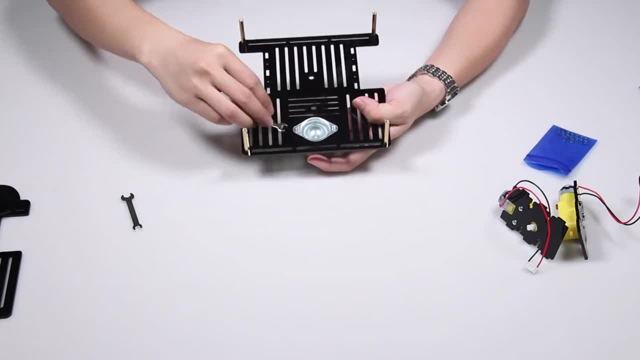 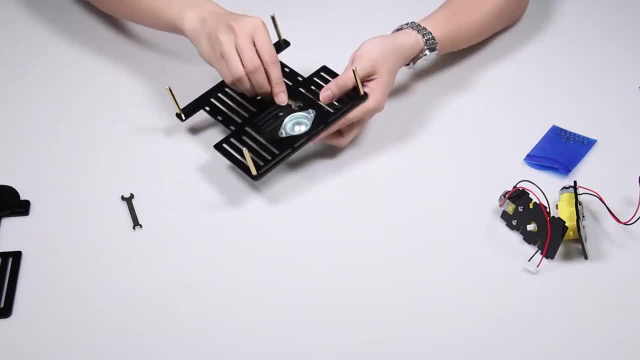 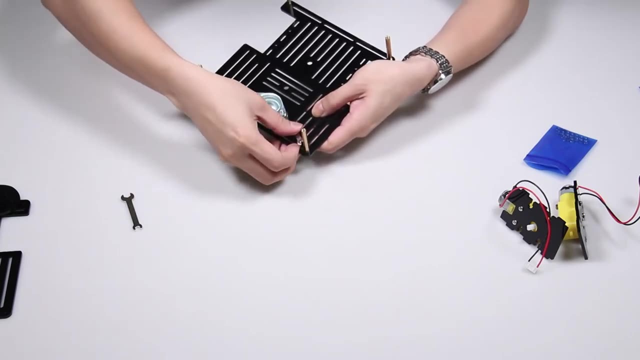 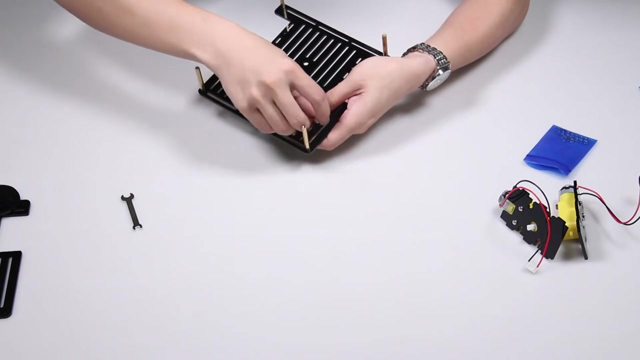 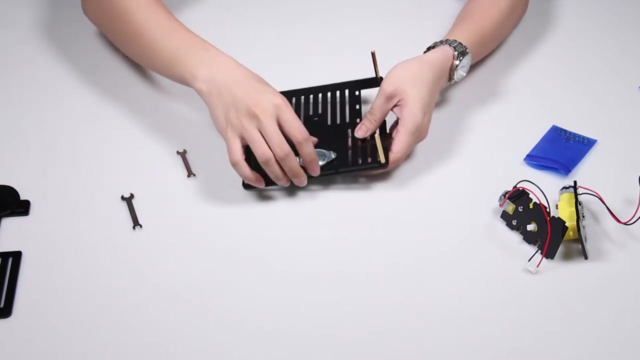 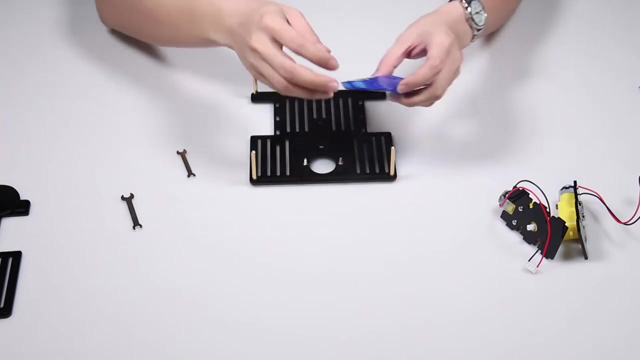 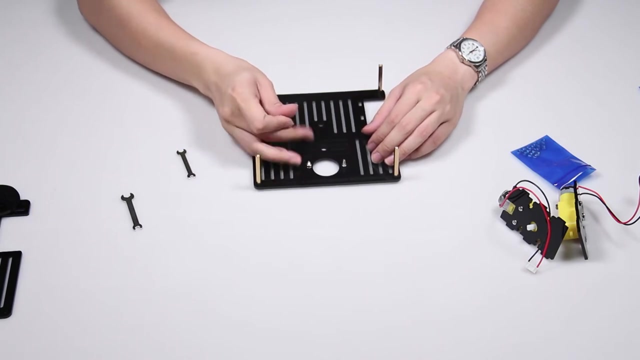 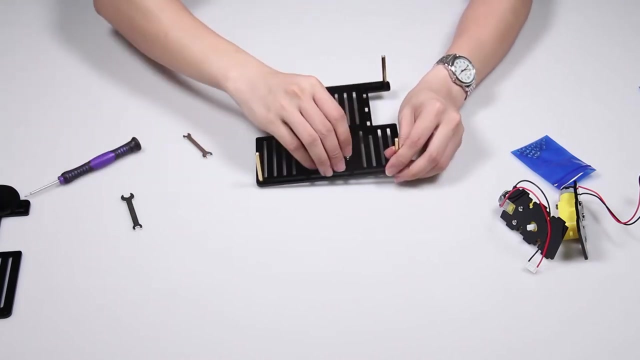 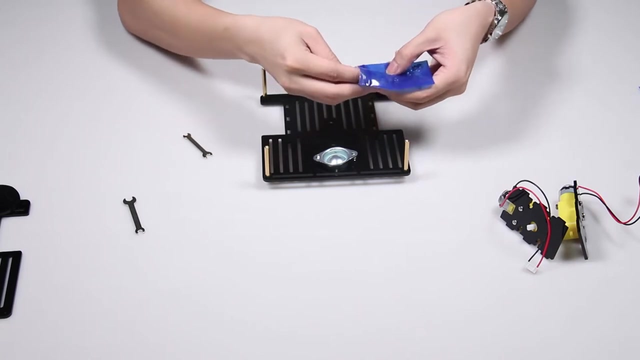 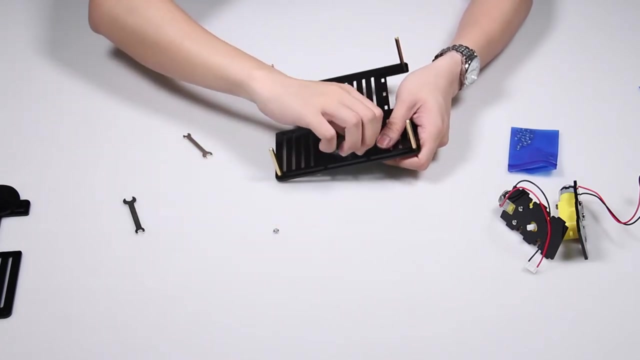 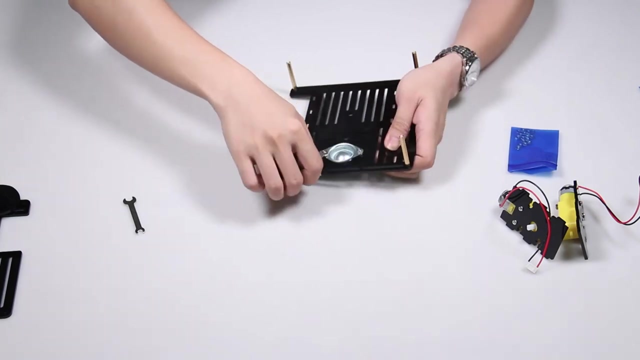 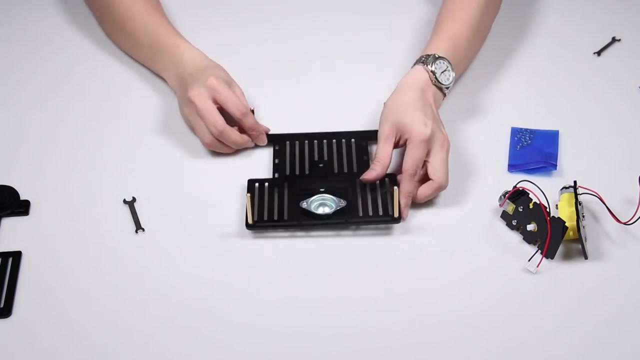 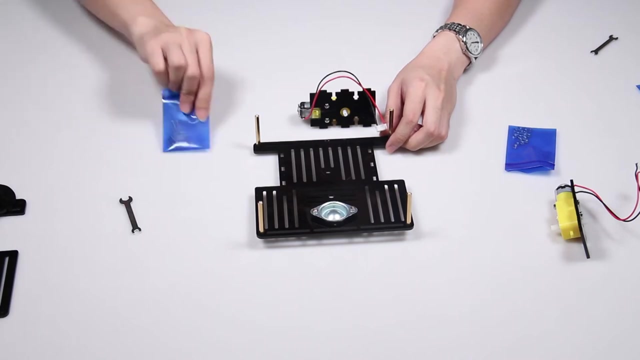 okay, now take off the universal wheel and mount two more nuts to balance the height. tight them as well. finally, put the wheel back on and fasten them with two nuts. okay, it's done here. now mount the motors onto the bottom plate with m3 10 nut screws and m3 12 screws. 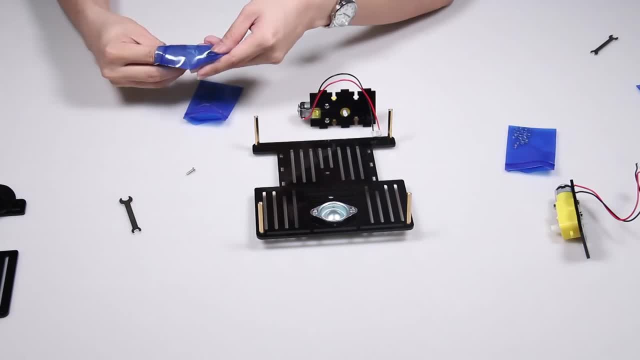 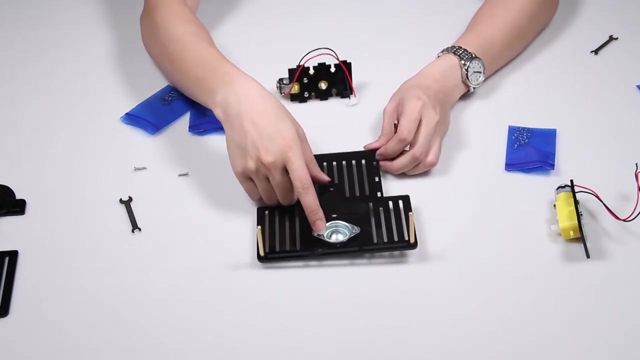 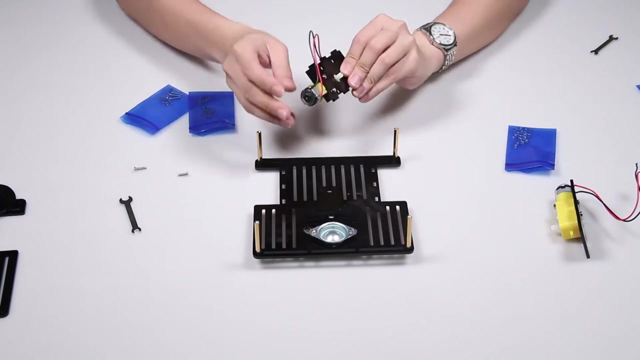 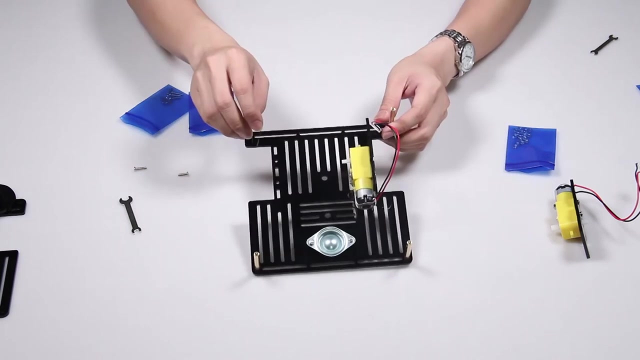 you can compare them: the longest one should be 12 and a little shorted one should be 10, like this, and here the universal wheel is the front wheel, so this should be the left wheel marked with L, and it should mount like this. I don't know how to describe this, but you can see. 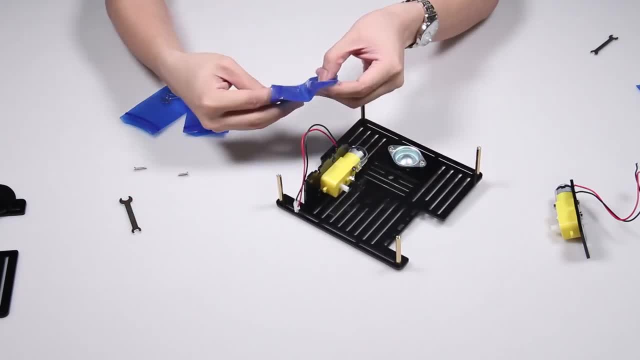 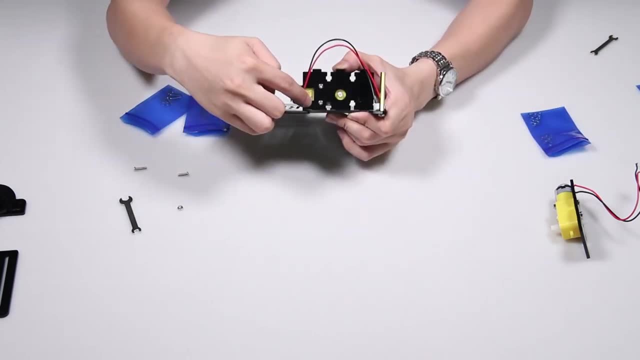 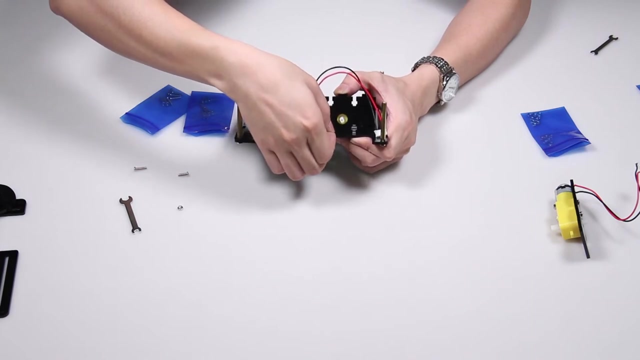 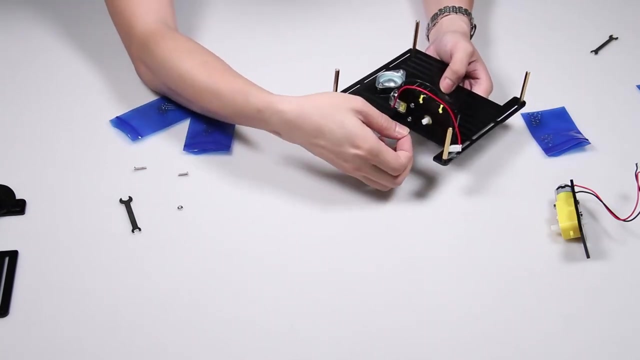 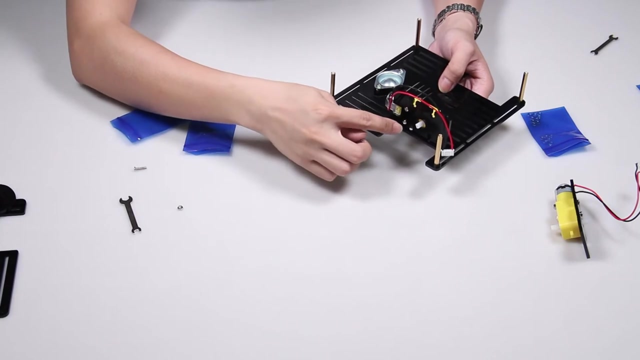 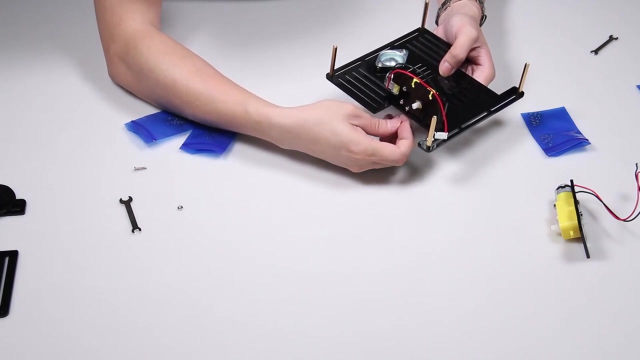 now put m3 nuts into the hole here here, carefully slide it in. maybe you should horizontal it like this and carefully slide it in and the short one- you can see the short one- should be the 10 and carefully put it on. let's try that again. 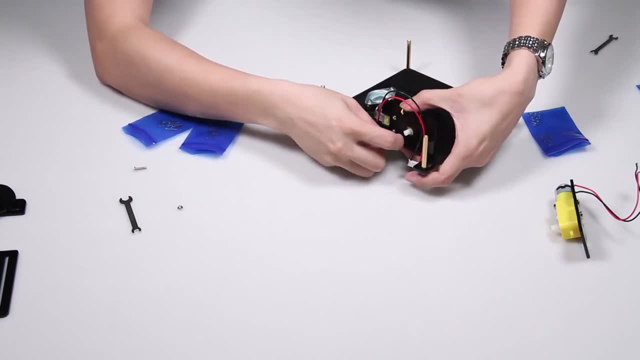 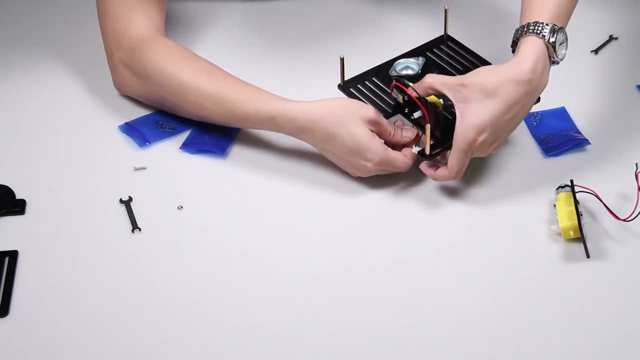 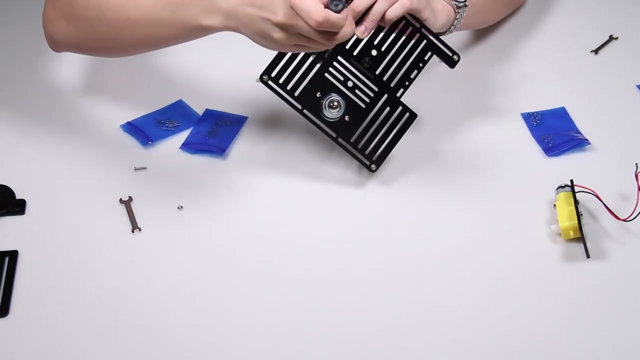 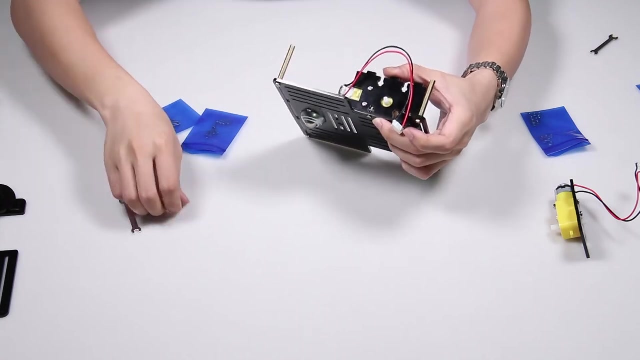 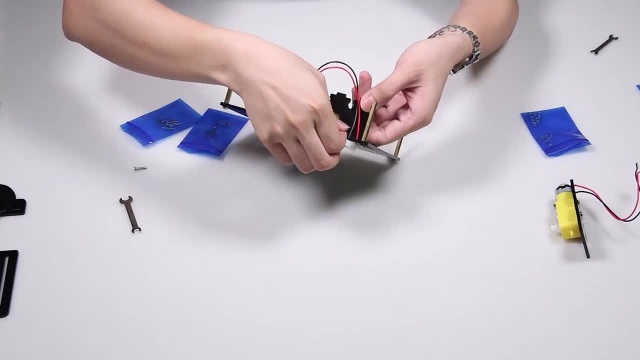 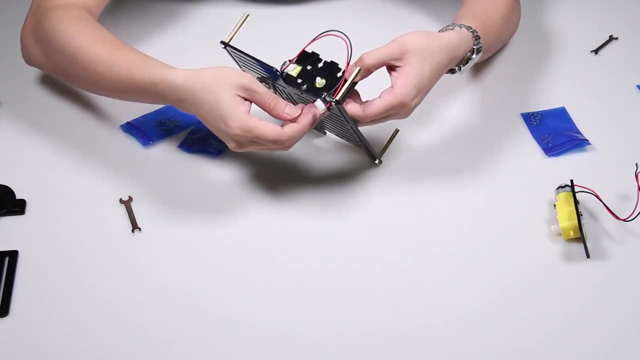 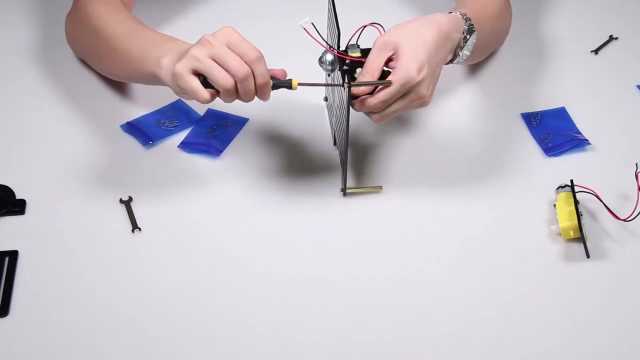 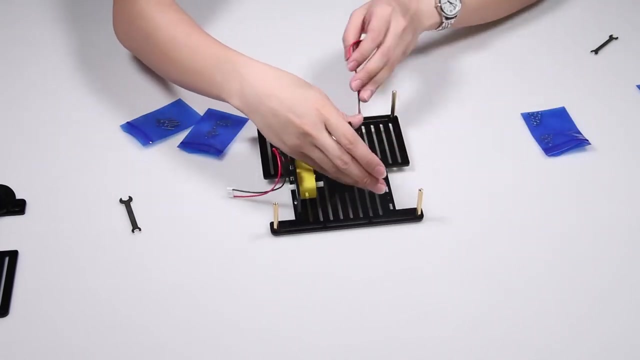 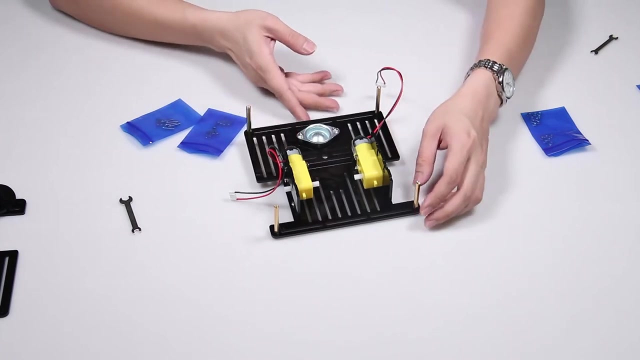 to press the nut, so the nut won't fall, and this way it would be much more easy. screw the 12. this is the wrong screw. okay, do the same with the other motors. and also it should be: look like this: the end should pointed it forward. also, mount it with. 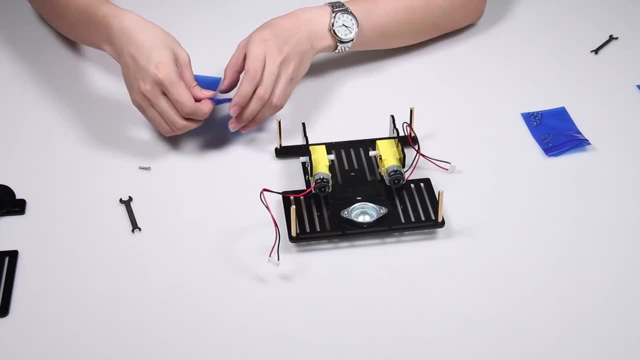 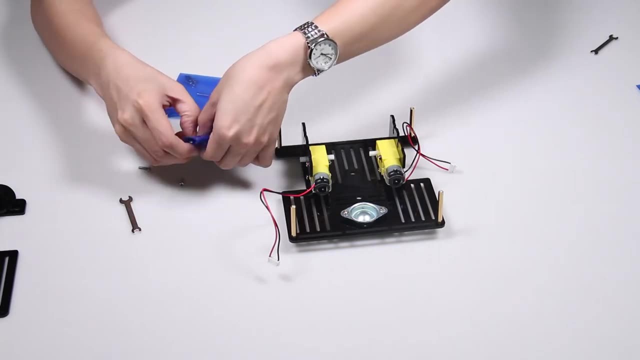 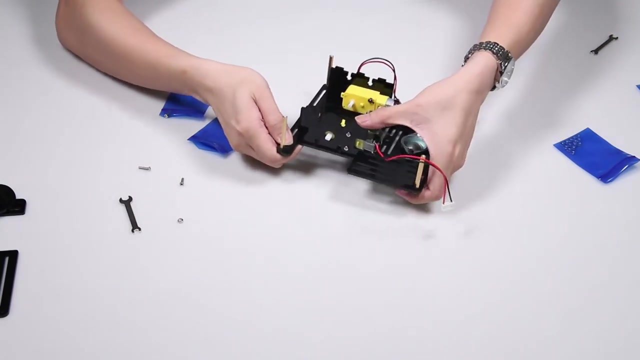 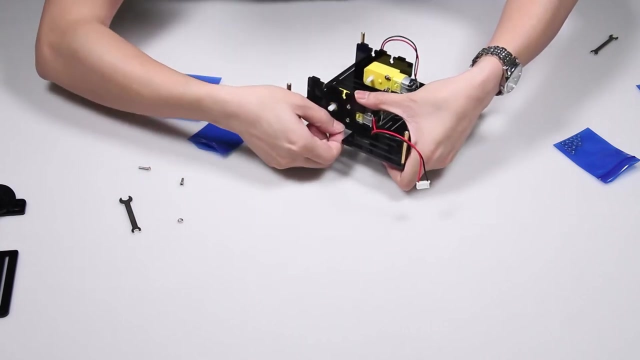 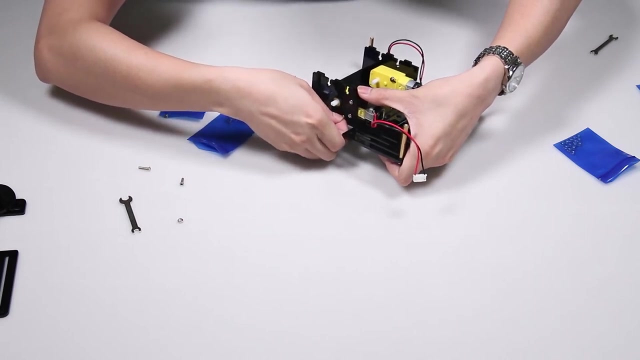 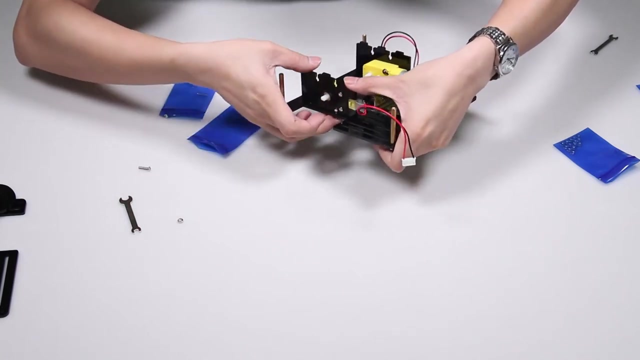 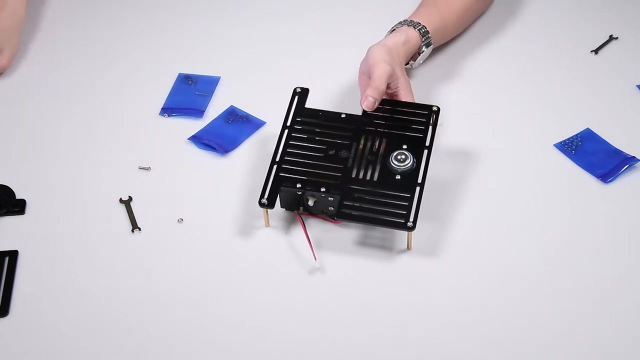 m3 12 and the m3 10, two nuts. okay, we will review this finger. push down, hold it horizontally and carefully insert the nut. put the m3 10 from bottom, press it, flip it and tight it. this one, this one. press your finger on the hole. 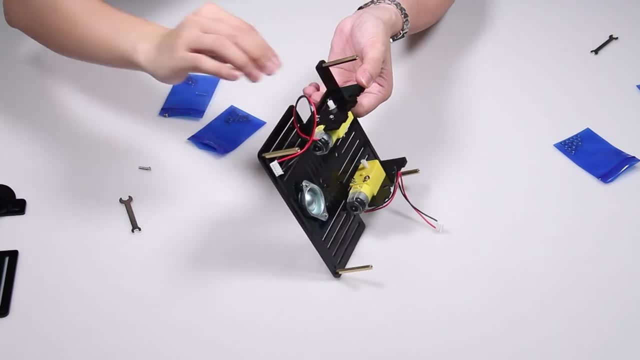 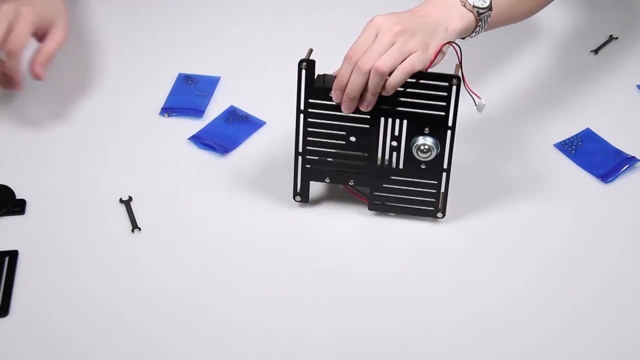 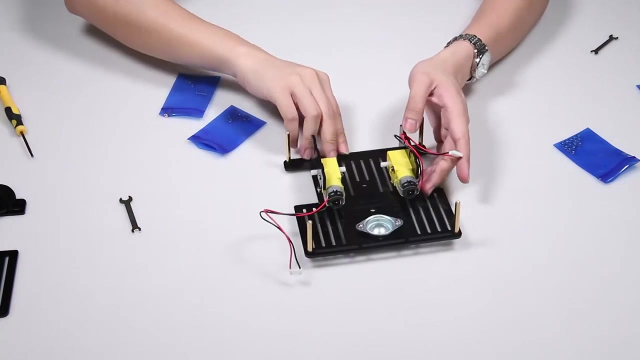 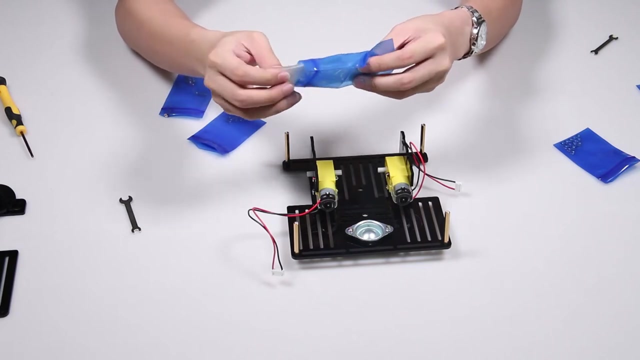 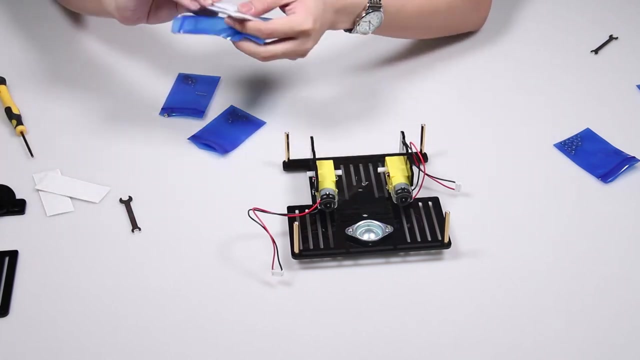 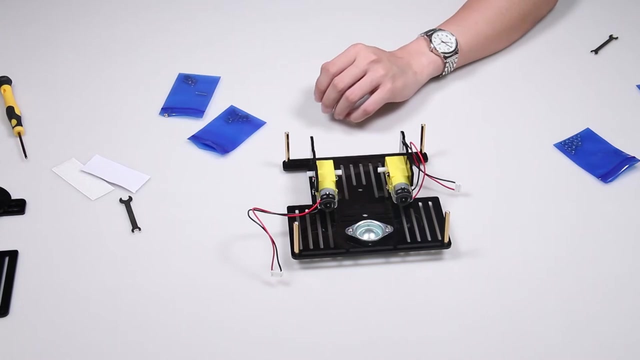 put the nuts in, then the screws hold it and tight it, then take a hook and loop tape and the nut and we'll do the same thing and take a look at this, this one, and take a look at this. look at this and take a see this. 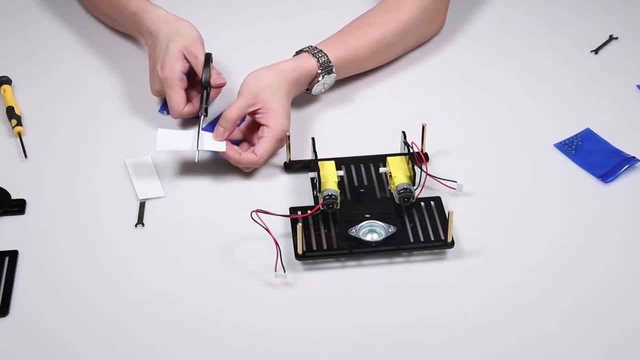 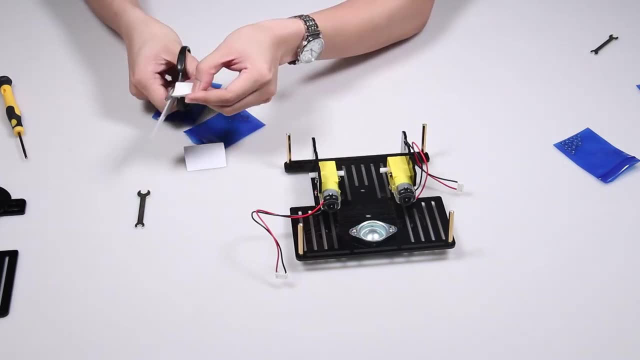 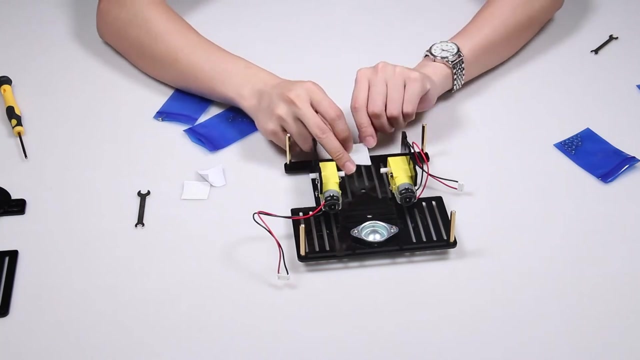 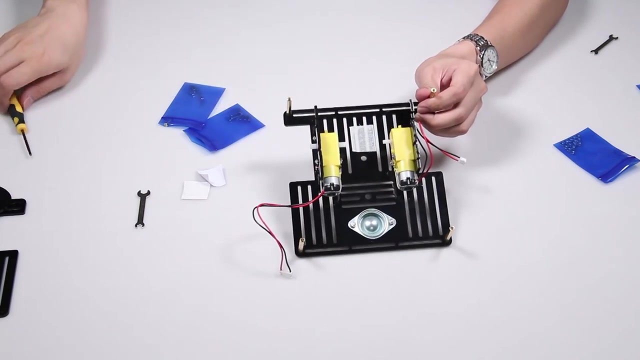 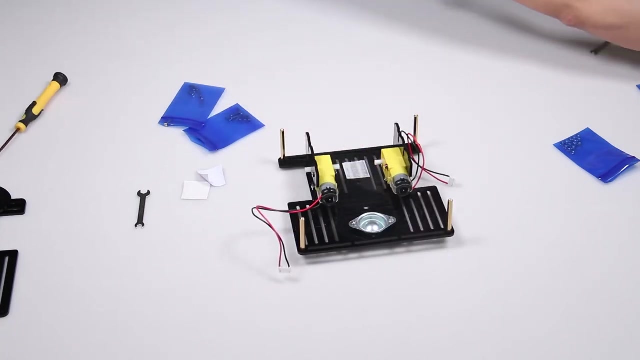 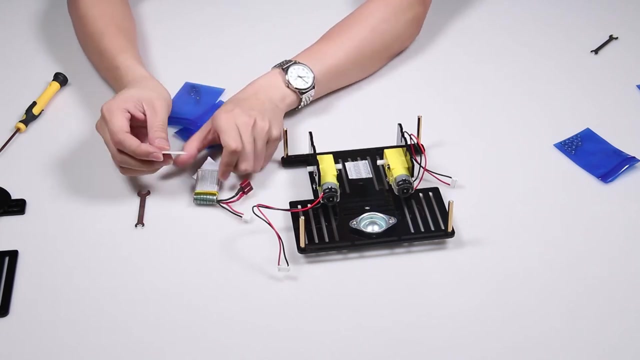 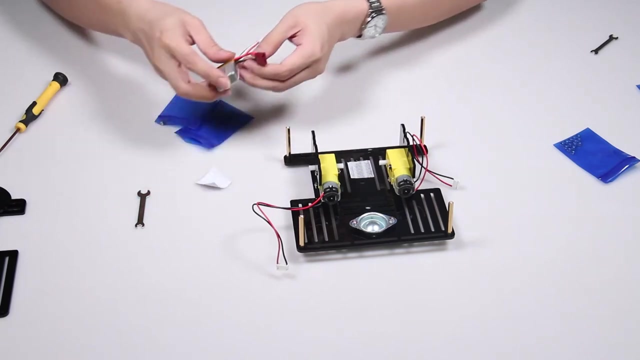 cut this like this lag this long, so it is to loop and stick the hook here in the middle, but not covering this round hole here. this is important. remember and stick the other one, the loop, onto the battery. I recommend, not the label size. okay, this way you can stick your battery here. 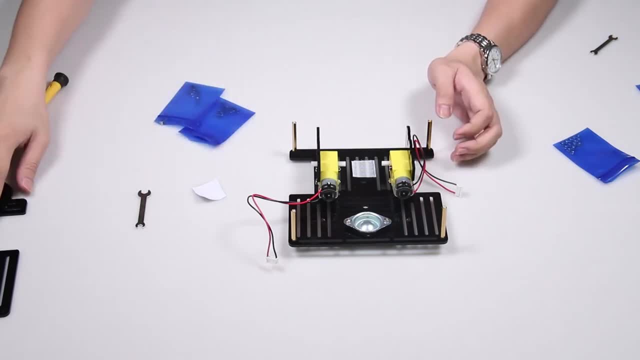 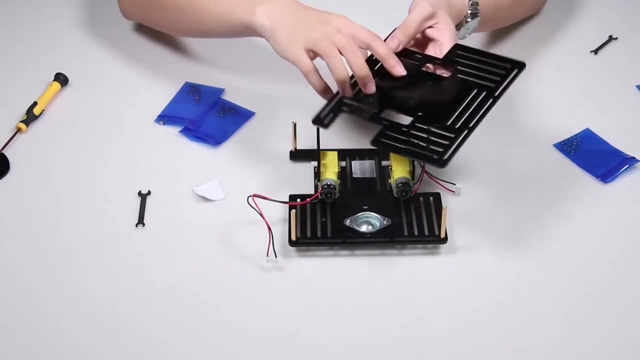 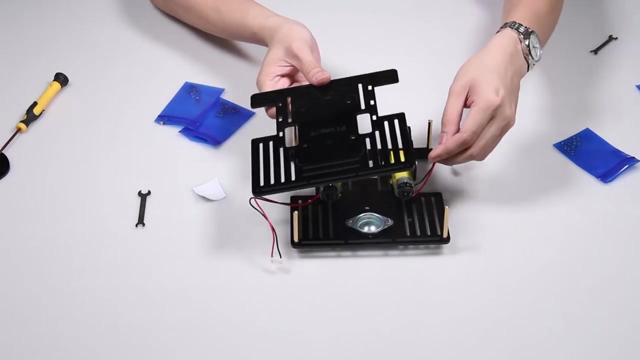 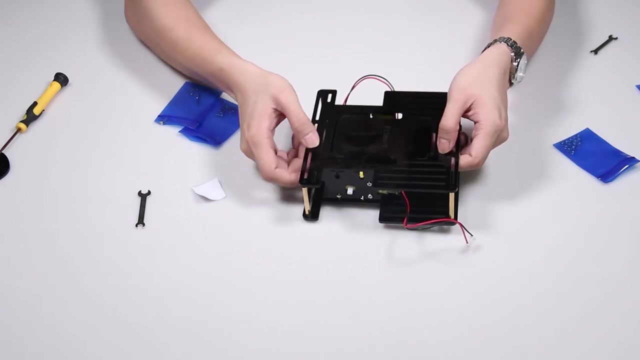 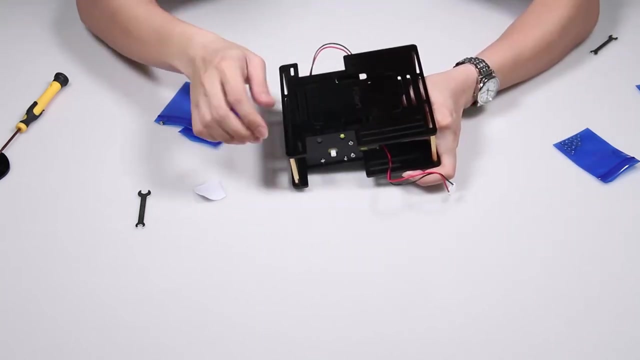 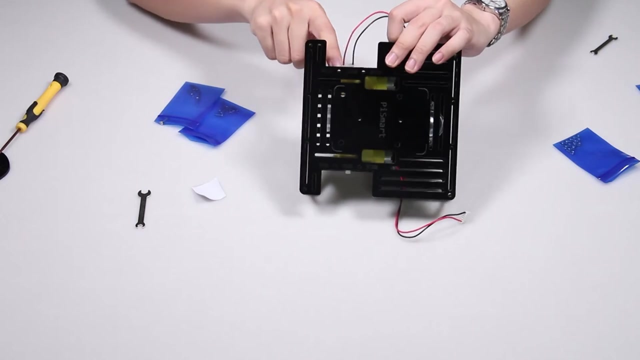 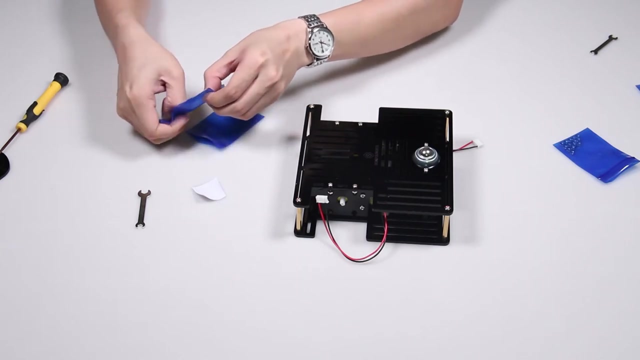 okay, to the battery aside. now let's mount the bottom board here. you should see a label here. mod pie smart should face up and you should put here and through these four, three blocks. okay, it should be flat like this. now mount the m3 12 screws. 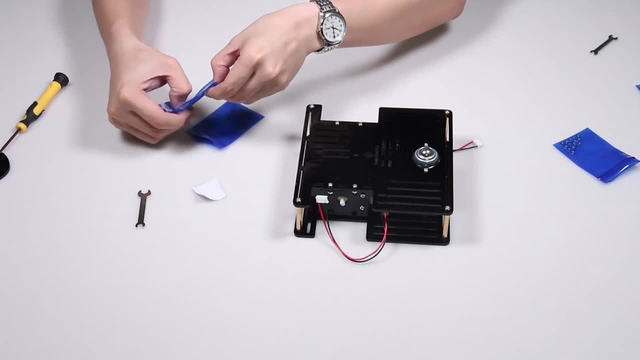 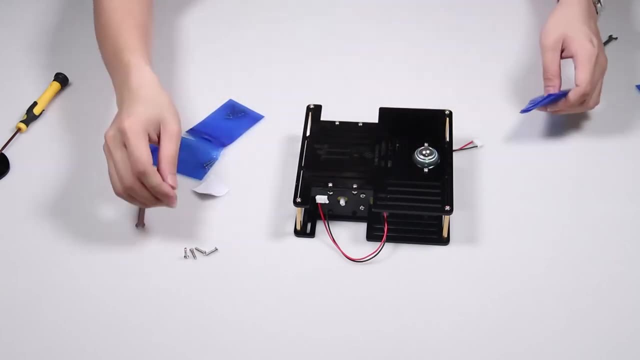 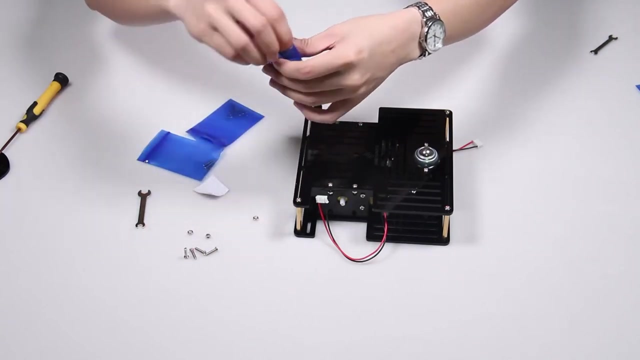 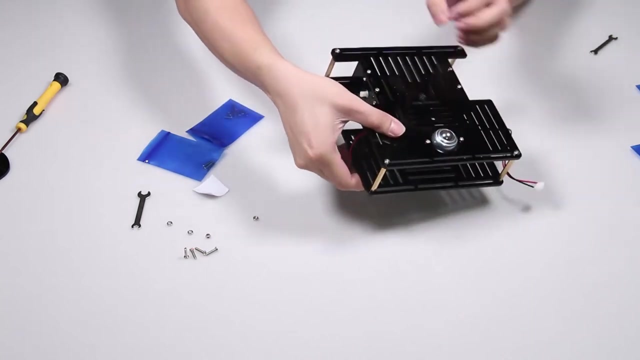 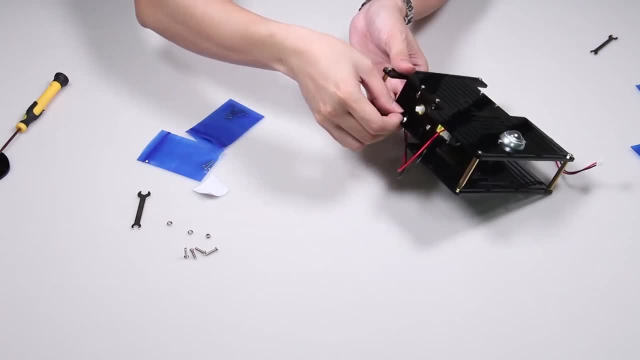 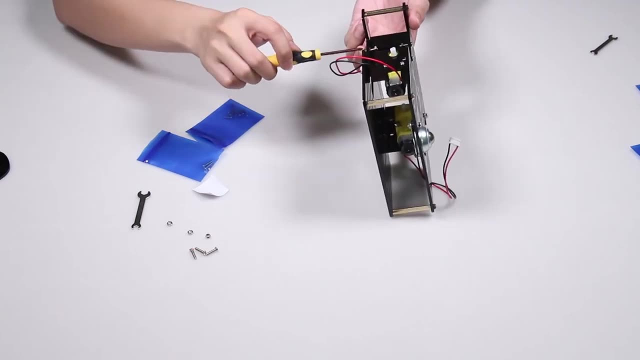 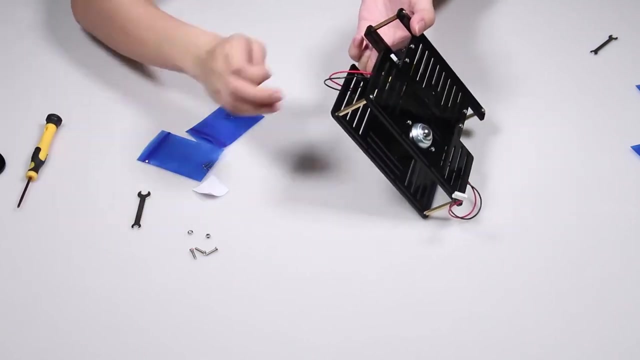 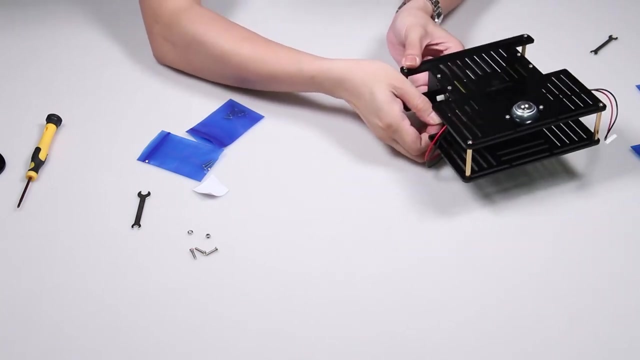 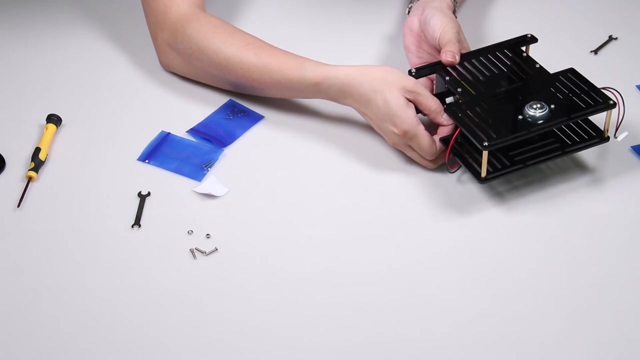 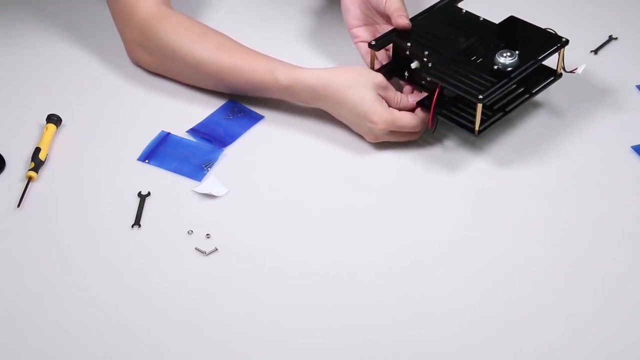 using this little stick to separate the thumb and the thumb here. hold the nut and the screws, tight them here too. if you can't fit your fingers in, you can just hold it horizontally, like what we did before, carefully, and put the screw from the bottom. you see it. 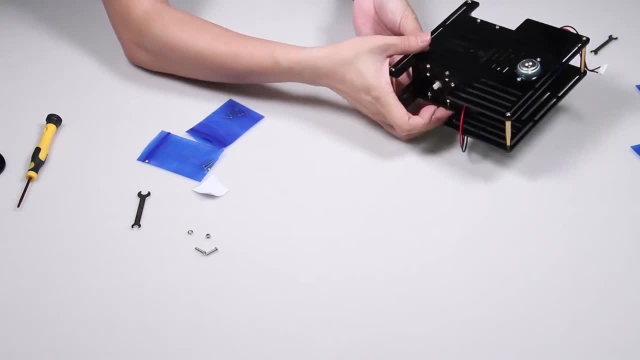 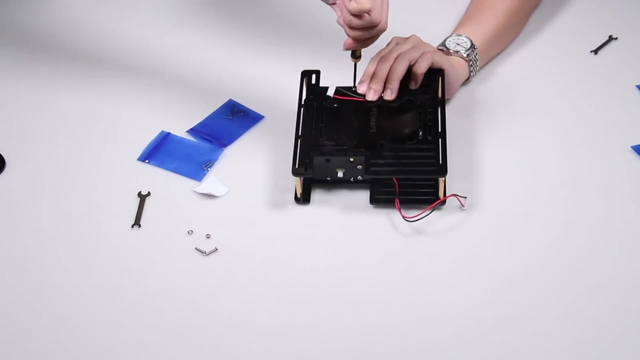 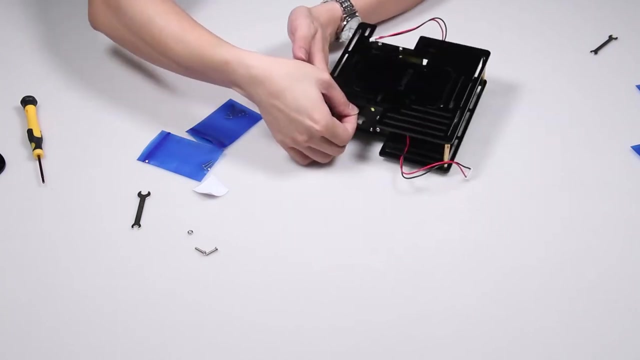 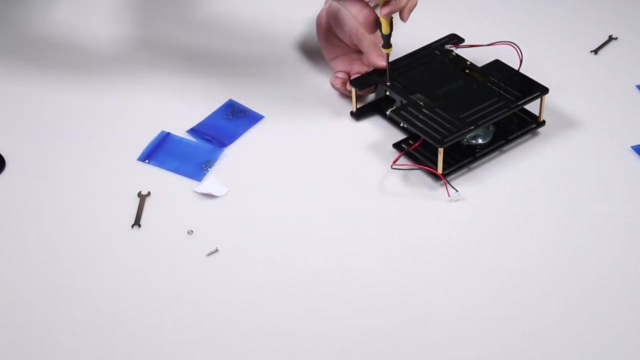 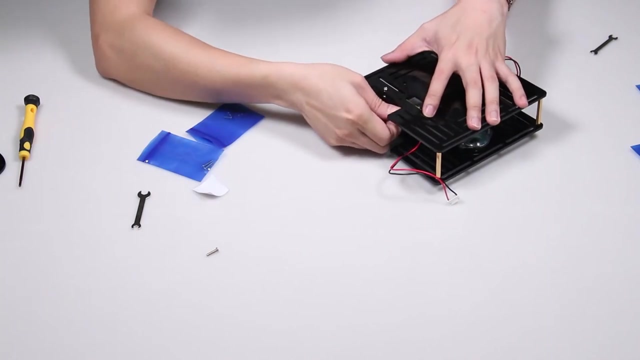 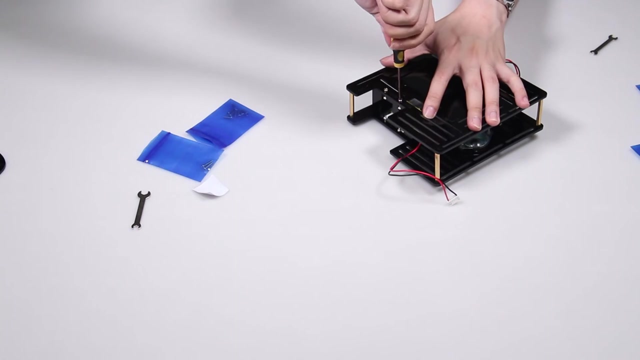 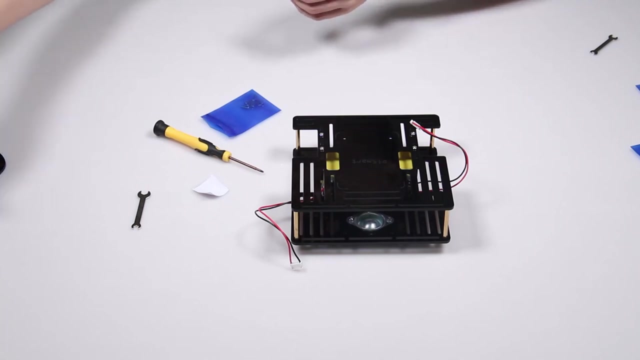 and press the nuts in case it move, and flip it and tie the screws. do the same here. maybe you can. you don't need to flip it just like this carefully- slide it in and put screws. this way may be easier. okay, now this aside, take the sorted screws, the m38 screws. 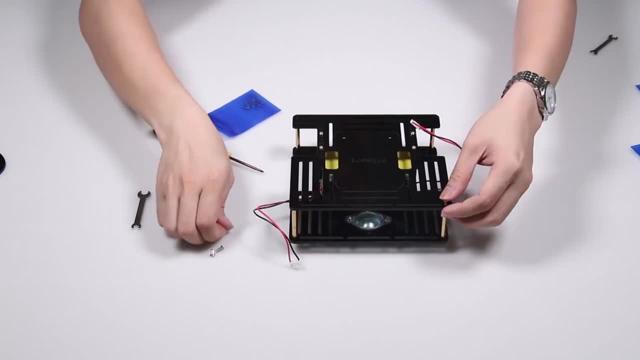 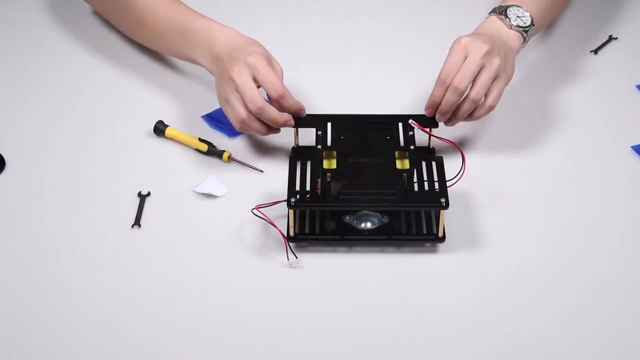 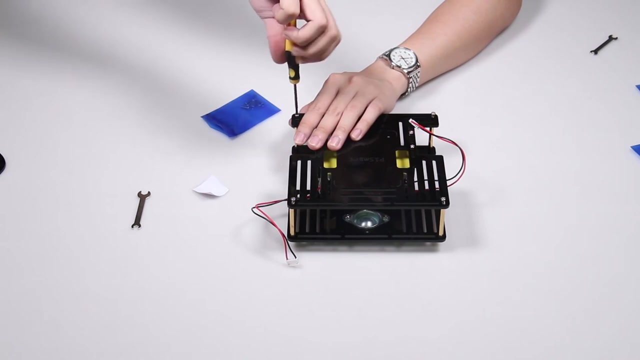 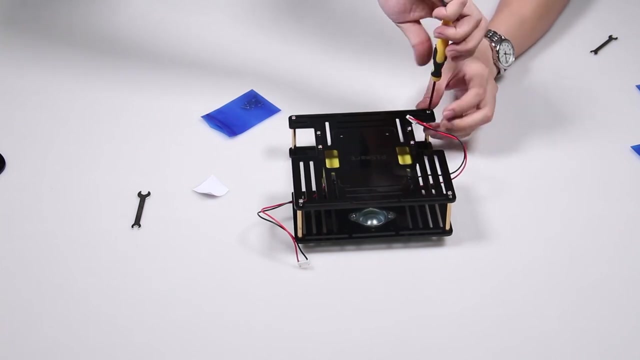 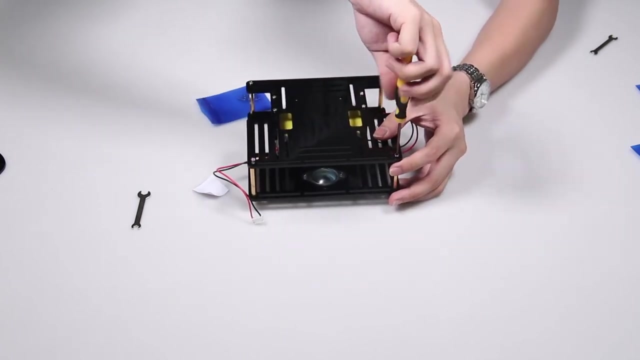 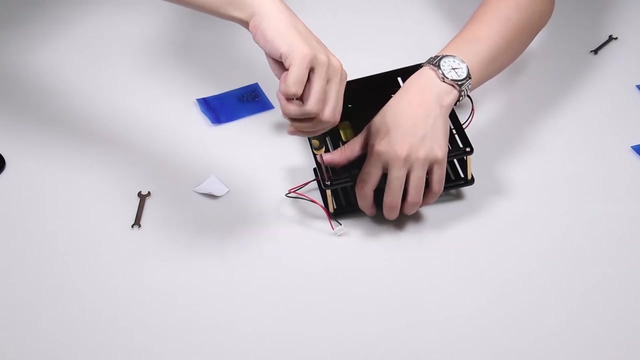 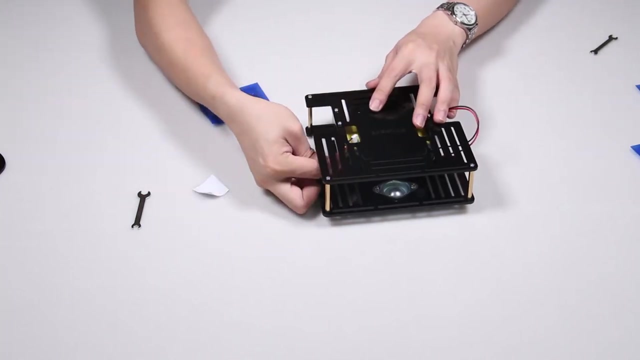 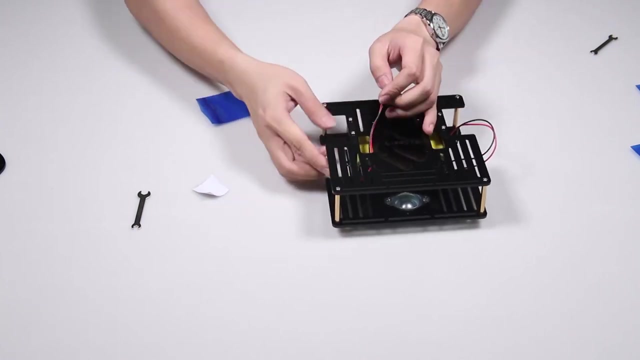 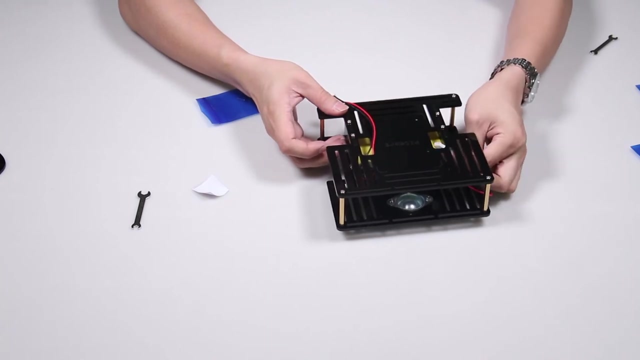 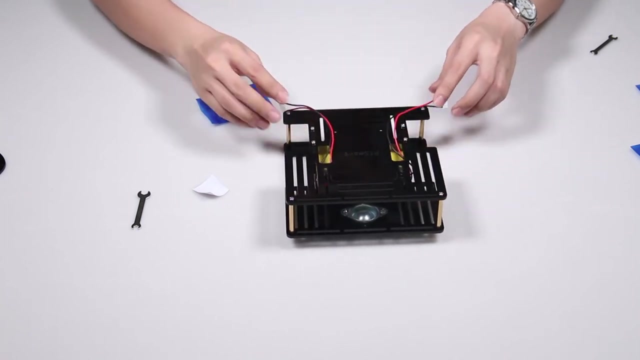 this should fasten the four corners with the copper standoff Tied, all four of them as well. Okay, finally, thread the cable through the hole. This should be in Like this: Thread the cable through the hole. Okay, almost done here. 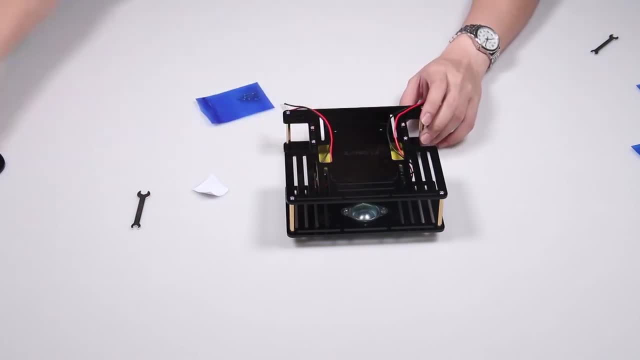 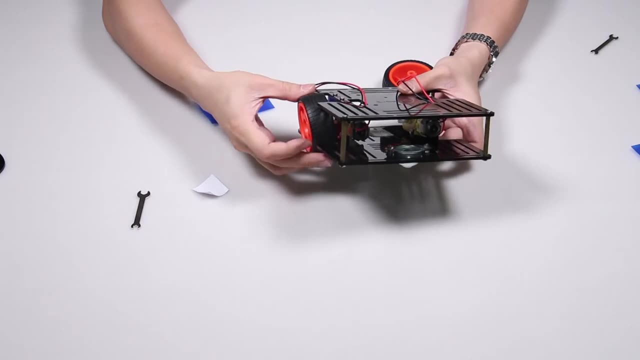 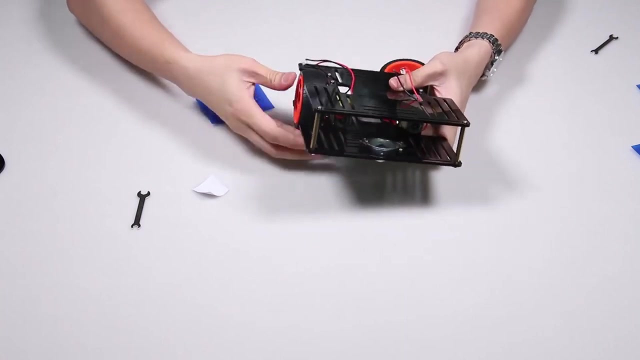 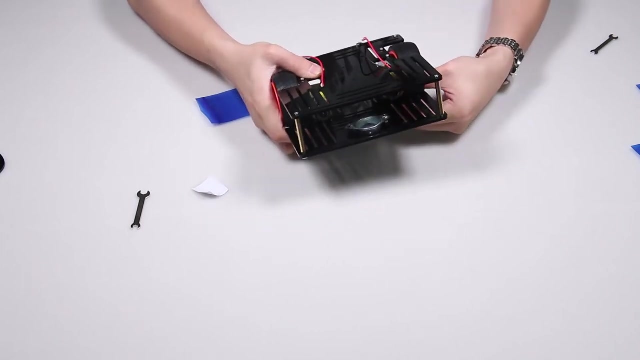 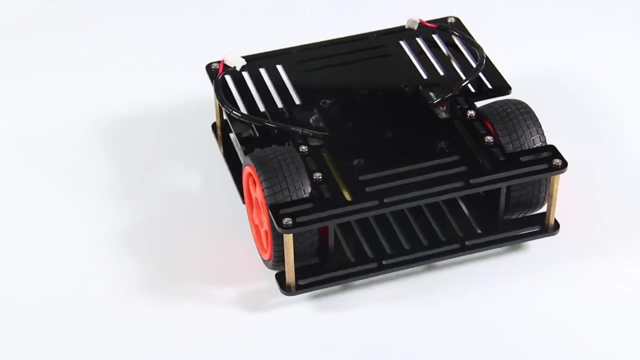 Sorry, I forget to put on the wheels. So let's take the wheels here and mount it here, Spin a little bit and push it in This wheel here too. Okay, now it's done, So you can mount the sensors now or whenever you need it. 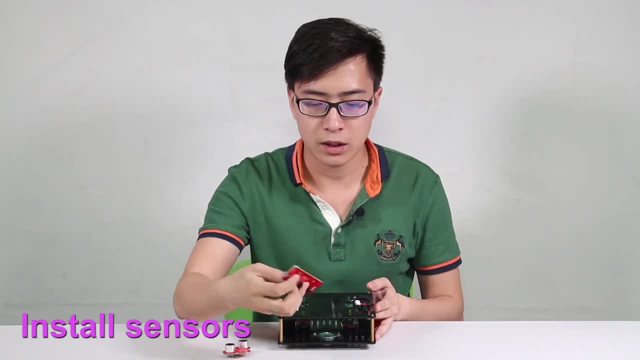 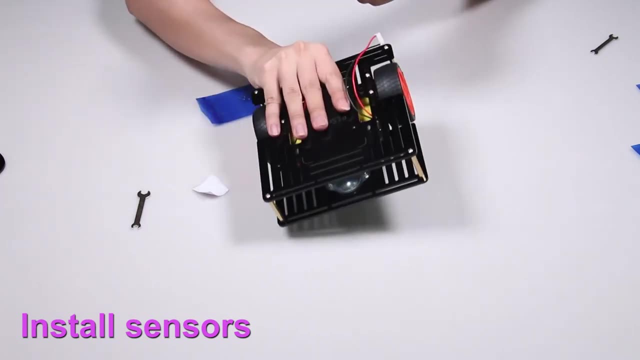 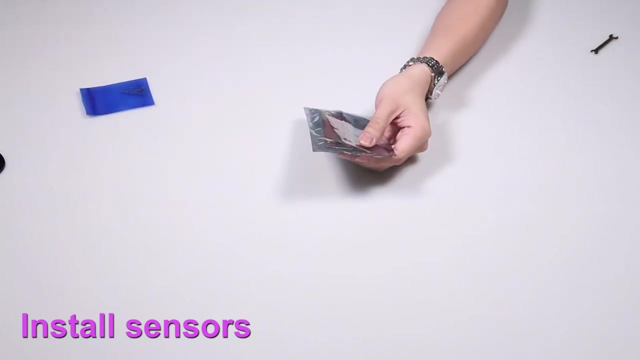 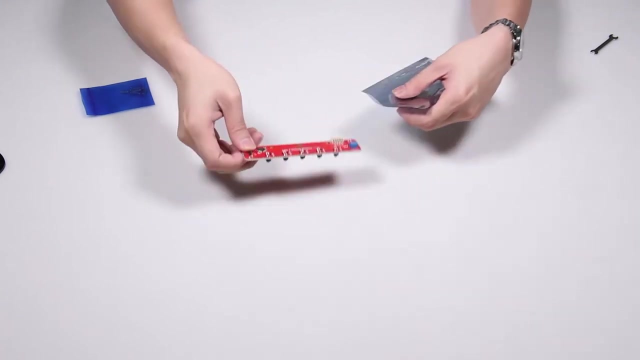 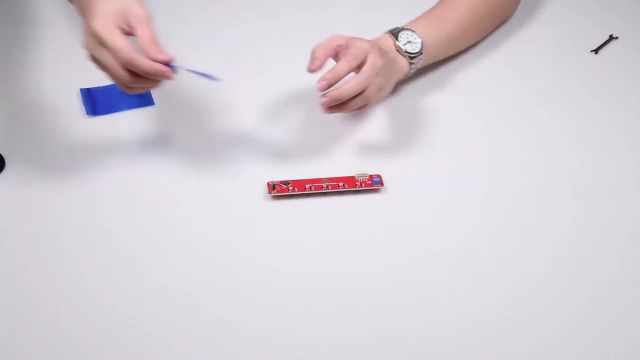 But I'm gonna just show you how to assemble the sensors. Now take the line follower. Put this aside first. Take the line follower- You can see the five sensors here- And take the M3 8 screws as well- 8.. 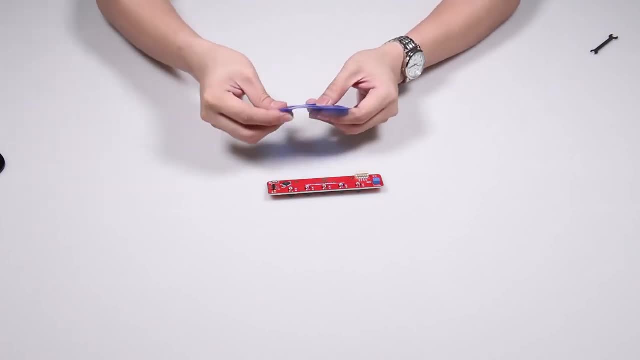 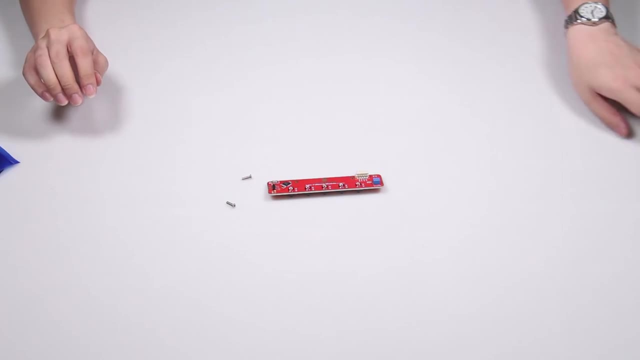 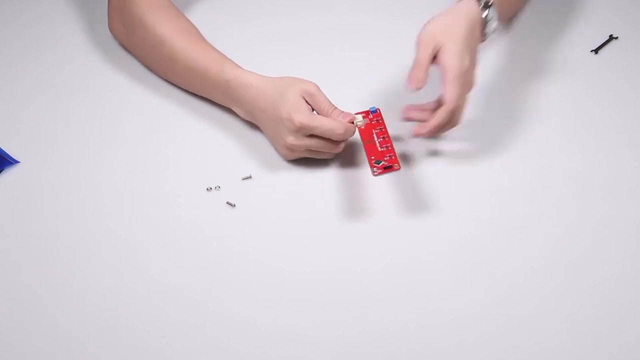 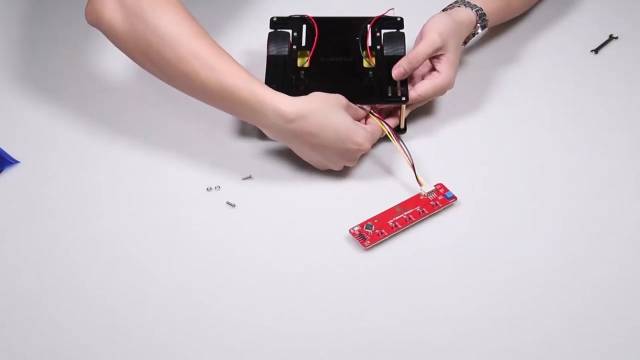 Should be 10.. M3, 10 screws And M3 nuts And the four-wired anti-reverse cable, Four-wired one. Connect the wire first And take the car, Just mount it here. Thread the cable first. 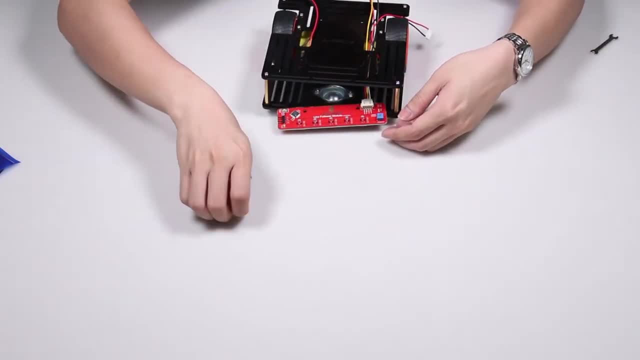 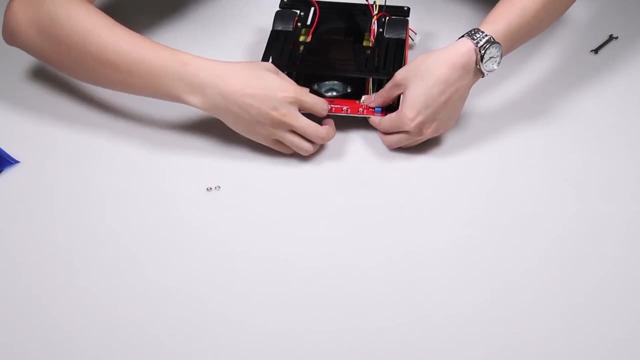 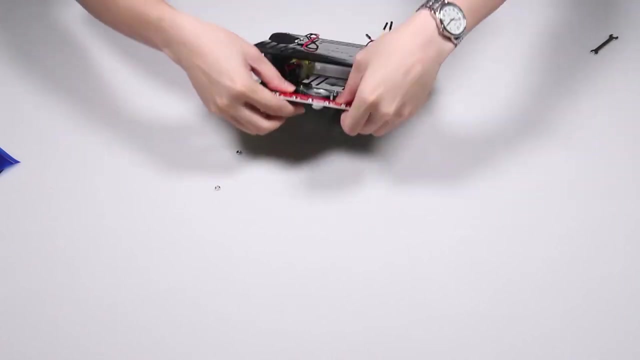 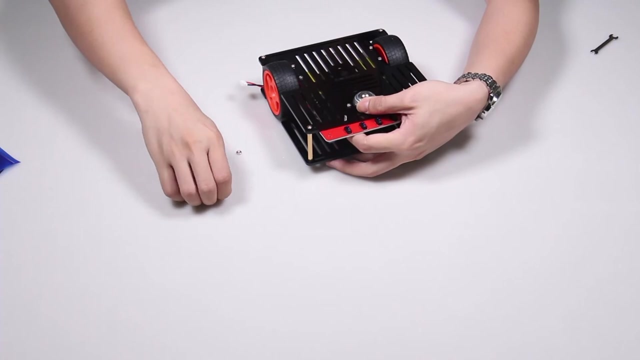 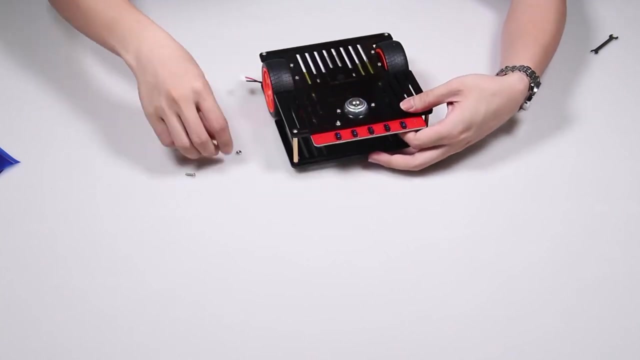 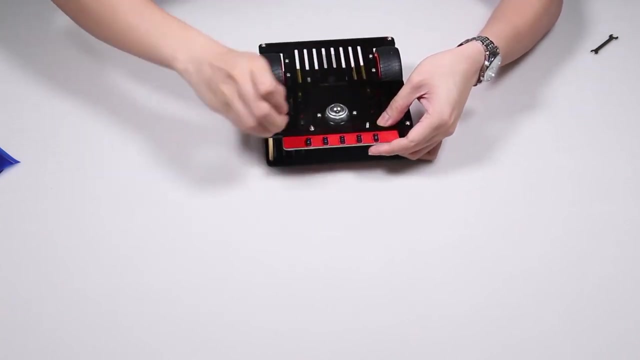 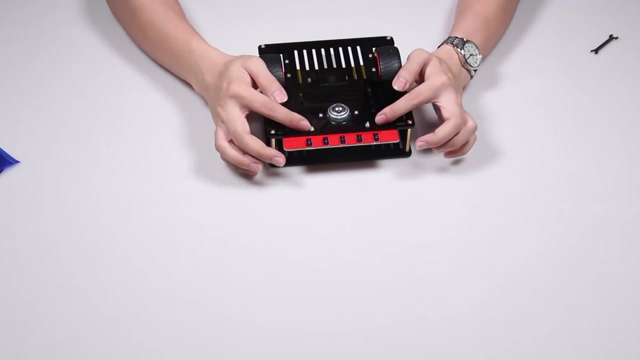 To the top And take the screws in, Okay, one by one, To the left, To the right, And to the left, And to the left And the right. okay, do not tie them first. you can see it's a slot. so align the center and then. 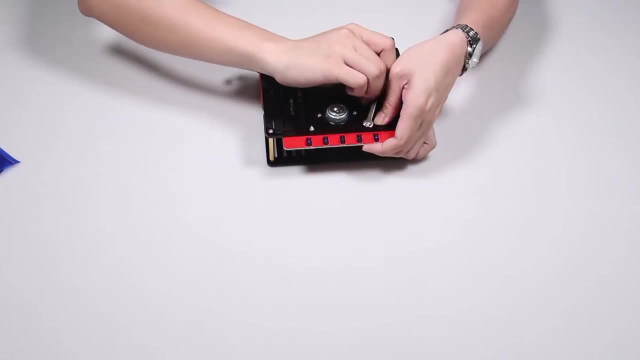 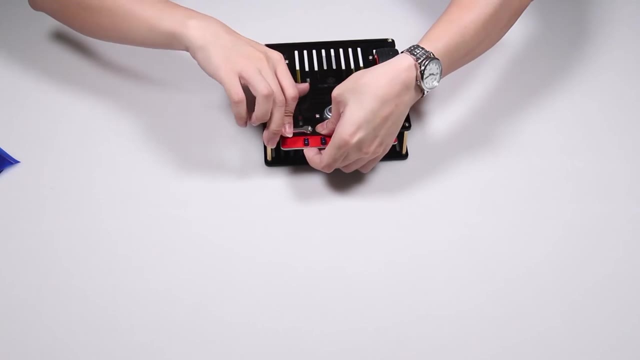 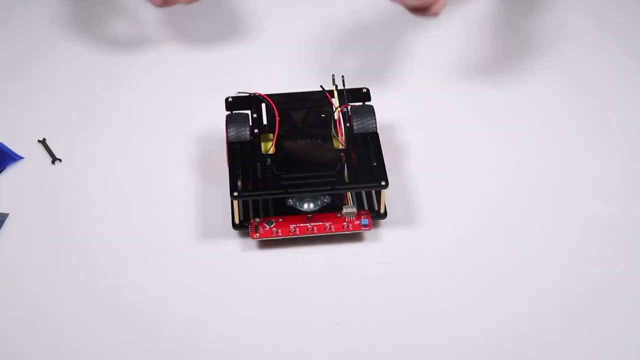 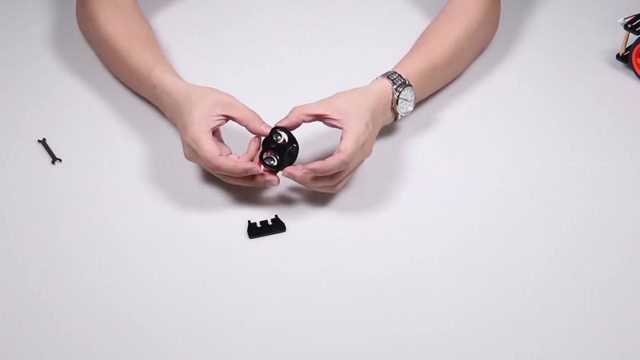 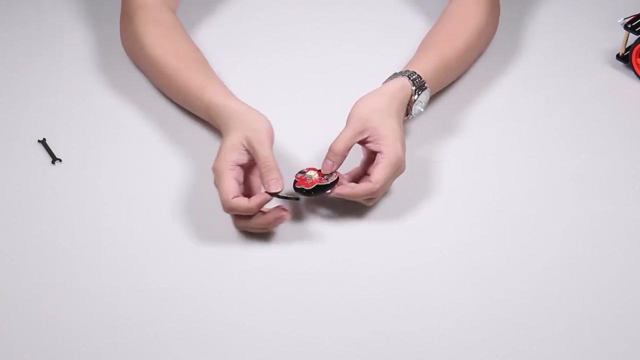 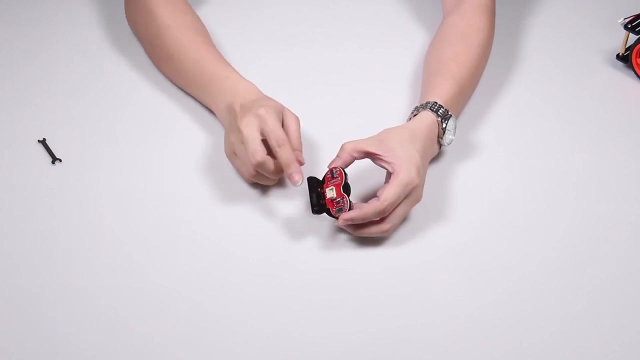 tie it. you can use the wrench or use the screws. okay, just like that. now install the ultrasonic sensors. this one, take it out and take the last two pieces of the acrylic. acrylic. mount it like this. put this on and turn it over and put this in a 90 degree angle, like this: 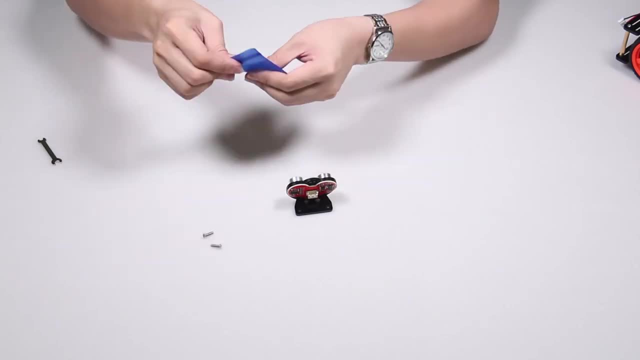 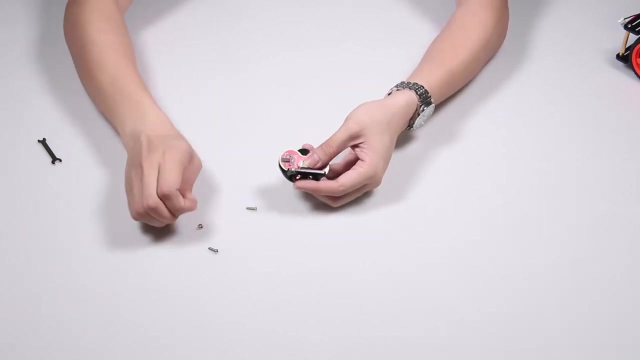 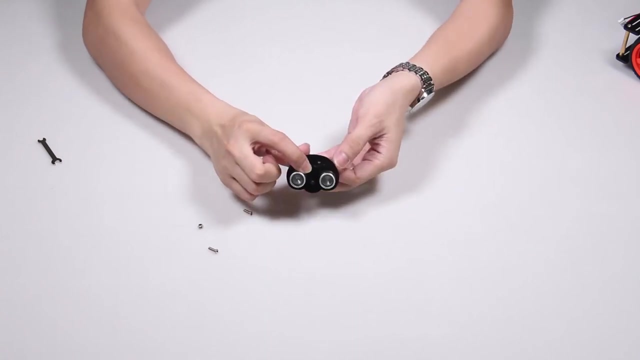 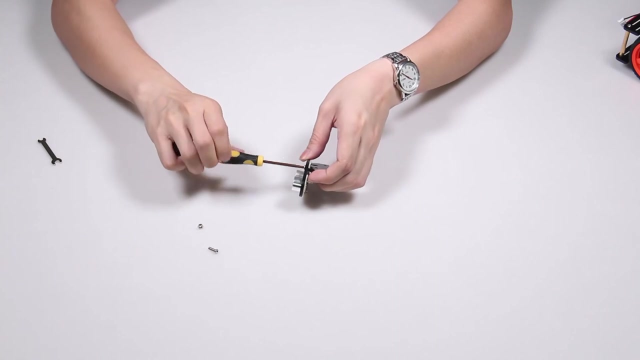 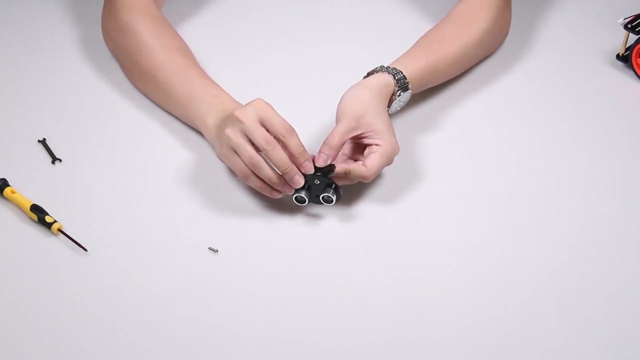 now take the M3 10 screws and the M3 10 screws and three nuts to fasten these. it's the same process: put in this screw, put in a nut. it's not easy this way. put in a nut and the screws off, Tied it.